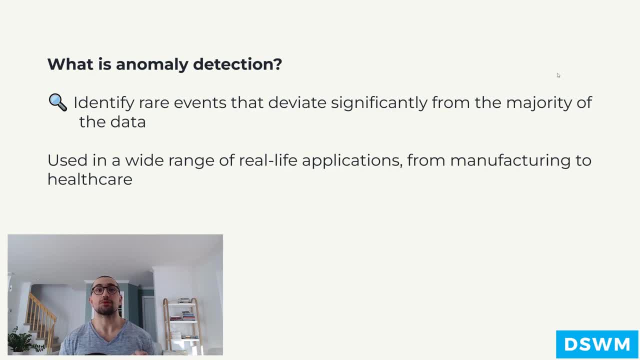 identify rare events that deviate significantly from the majority of the data, And it's very useful, right. It's used in a wide range of real-life applications, from manufacturing to healthcare. And now, why would you do anomaly detection at all? Well, for two reasons. First, 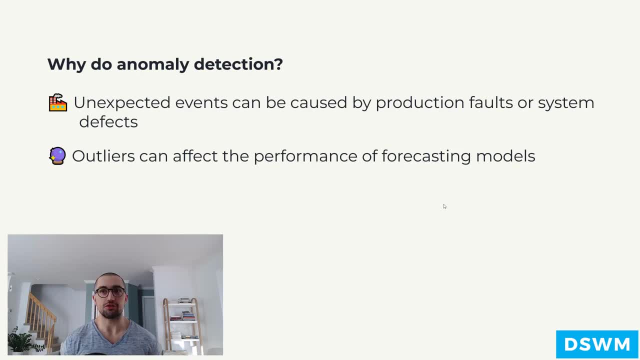 unexpected events usually are caused by some kind of production faults or system defects, right, And it's very important to identify those. So, for example, it might be that you have a problem with your internet connection, For example. imagine that you're working at Amazon. 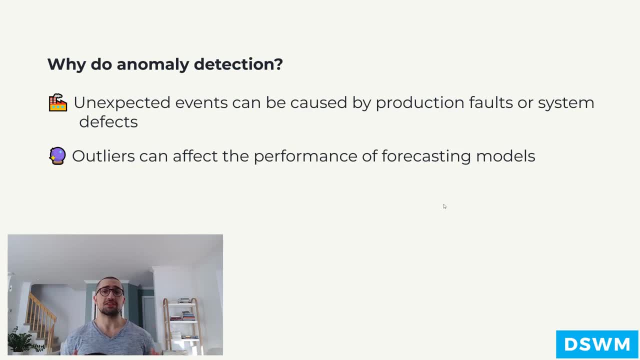 right, And you're monitoring the number of visitors to the website. Well, if, at any point, the number of visitors falls to zero, clearly something is wrong. right? Maybe your website is down, and so you need to identify that as fast as possible so that you can fix it okay. 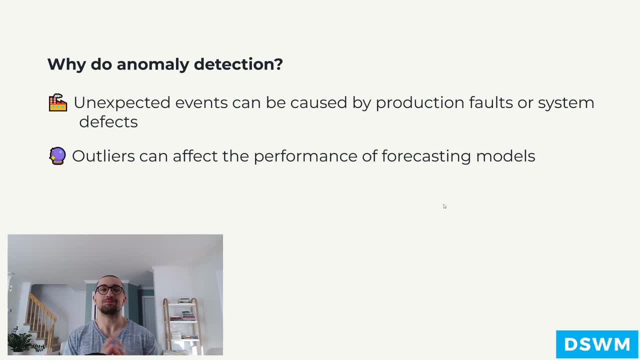 This is a pretty extreme example but you understand. you know why we would do anomaly detection. And the second reason is that outliers can actually affect the performance of your forecasting models. So we know that in time series forecasting model uses past values to then predict the future, right? So if in 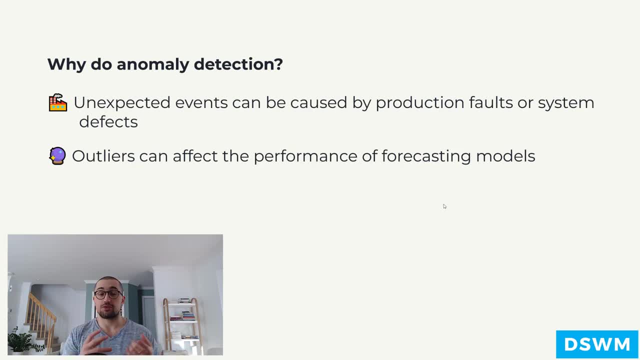 your past. you have some kind of outliers. well, you need to first identify them and then think: do you want those outliers to remain in your historical data, to turn your model on right? Is it reasonable to keep them? Should you remove them or try? 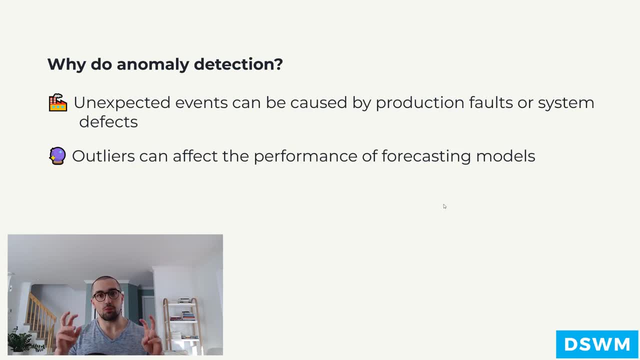 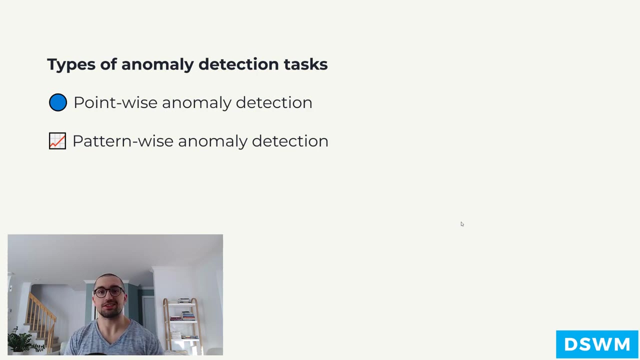 to normalize- you know their values- to bring it back, you know, to more normal behavior, in a sense, so that your forecasting model is more stable in the future. okay, So this is really the two main reasons why you would do anomaly detection. And now, like I said, there are two types of anomaly detection tasks. 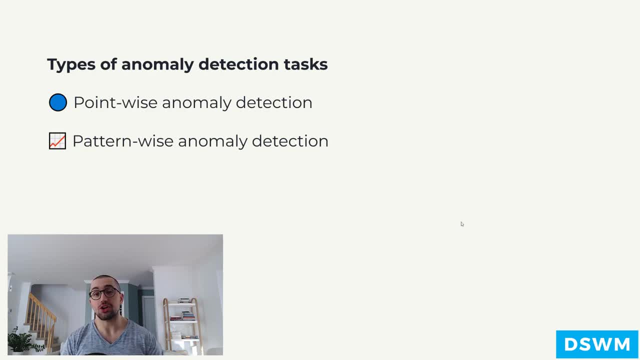 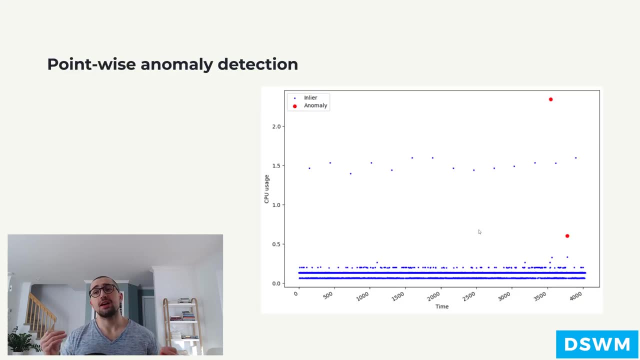 that you can do with time series data. The first one is point-wise anomaly detection and the second one is pattern-wise anomaly detection And they're pretty self-explanatory. so point-wise, as it says, you know you are looking at isolated points in time that are outliers. So here you can see an. 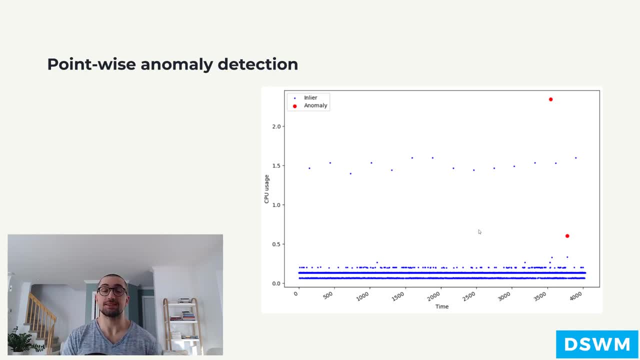 example, This is actually the scenario we'll be working with in this last slide. So this is actually the scenario we'll be working with in this lesson. It is the CPU usage of an AWS EC2 instance. So, as you can see, those two. 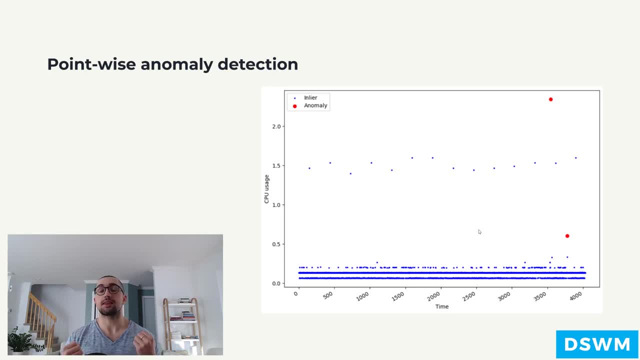 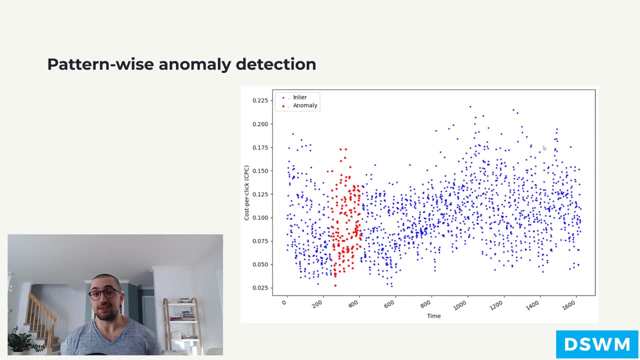 red dots in the time series. they are two isolated anomalies that were labeled, and so we are interested in identifying them. okay, And then for pattern-wise anomaly detection: well, here you are looking to identify a sequence of points that form an anomalous pattern. okay, So here again in our data, we have another scenario. 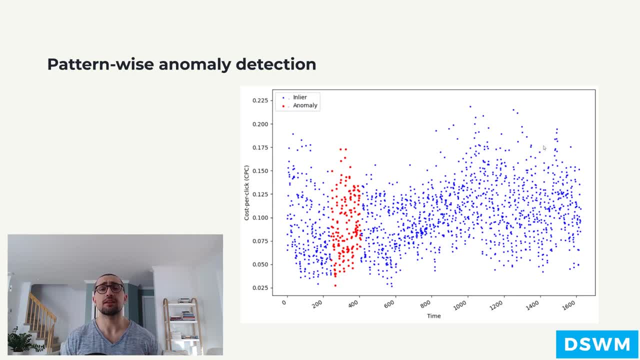 here, where we are monitoring the cost per click of an ad, and now you can see that the series of red dots is considered to be abnormal. okay, And so you would have. you would use other algorithms to identify this entire sequence of anomalous points. But, like I, 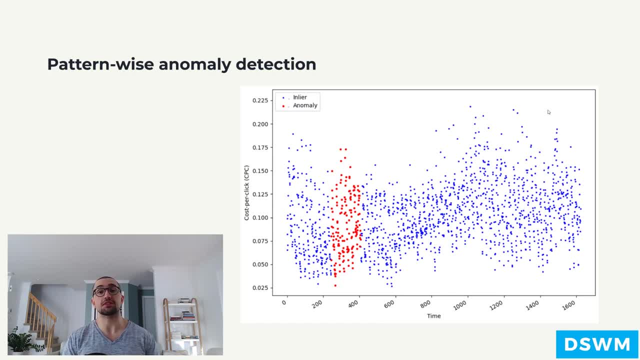 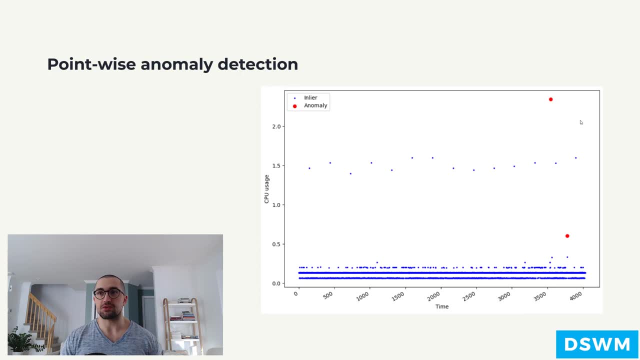 said, for this lesson in particular, we will only focus on point-wise anomaly detection. So this is the previous example, right, We'll try to find. can we devise, you know, algorithms that are able to identify these two red dots here? 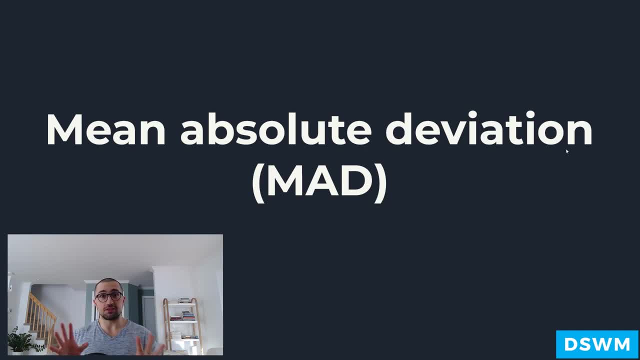 Perfect. So that's it for this little introduction. So before we actually move onto the first method, let me go back into the code. right, We'll read the data, import it, visualize it a little bit and then we'll come back to the slides and 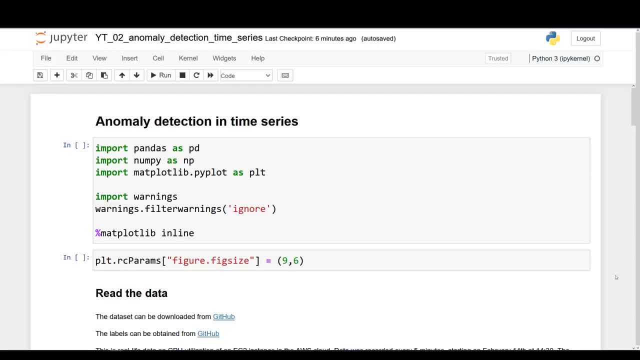 learn about our first method. Alright, and we are in the Jupyter Notebook. Note that you can get this exact same code in the description. I will leave you a link to the github repo. For now, we are just going to import out ouriles library. Let me just make a note that this one is in the jupyter youpd. jupyter, I think you're all sparky in the sense of these fields, right, You get other elements where you have multiple Schrub, you get multiple objects, but I'm simply going to simplify over the time and kind of organize this paradigm for the scenarios. great, I hope you guys enjoyed this. Goodbye. 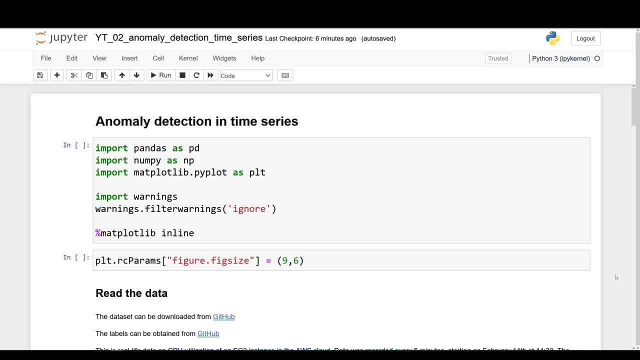 our data, read it and visualize it a little bit, and of course, i am not writing the entire code from scratch, because some parts are very boring, like you know: library imports or plotting. i really want to focus on the anomaly detection techniques, so let's go ahead and run these first two cells. 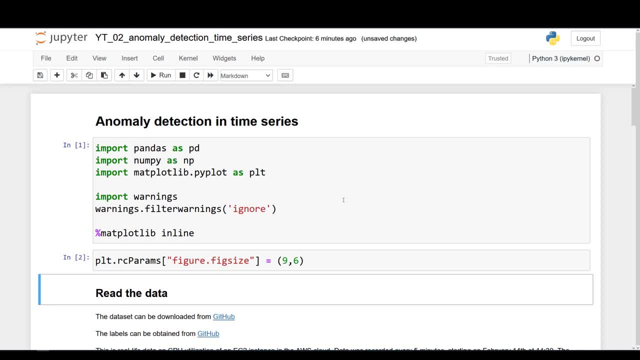 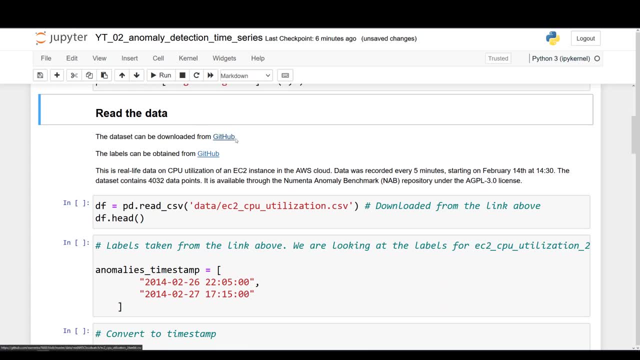 so again, i'm just importing the- uh, you know normal libraries that we use in data science. pen does not buy matplotlib, and then i am setting the size of my figures now here. this is where you can download the data set so we can use the exact same data as i am, so that you can reproduce all. 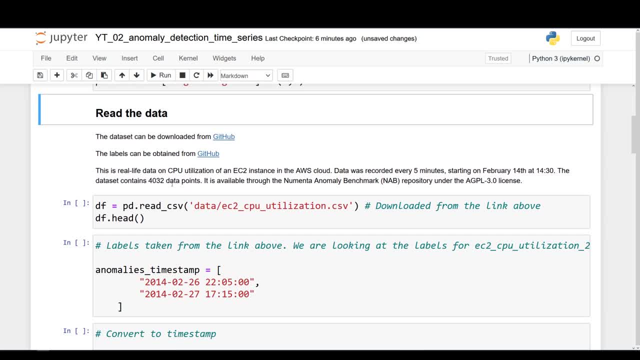 the results. so anyway, a bit of information on the data. you know it's real life data on the cpu utilization of an in situ ec2 instance in the aws cloud. data is recorded every five minutes, starting on february 14th at 2: 30 pm. there's a total of 4032 data points and it's made available through 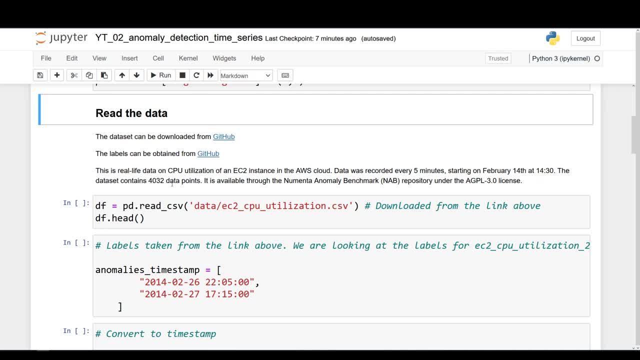 the numenta benchmark- anomaly benchmark, sorry- which is very cool repository and you have a lot of data sets with anomalies and the labels as well, and you can do either point wise or pattern wise anomaly detection. it's really cool, really, really grateful to have found this little repo there, so make sure to check it out and, you know, try. 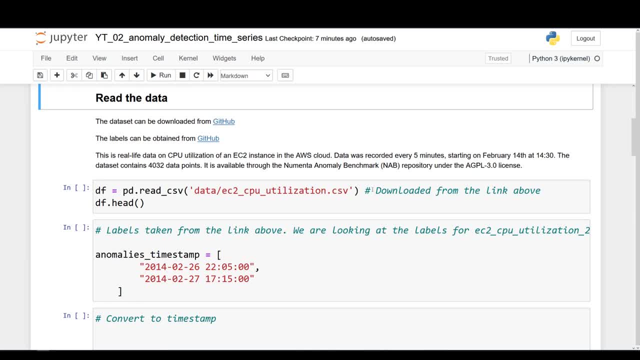 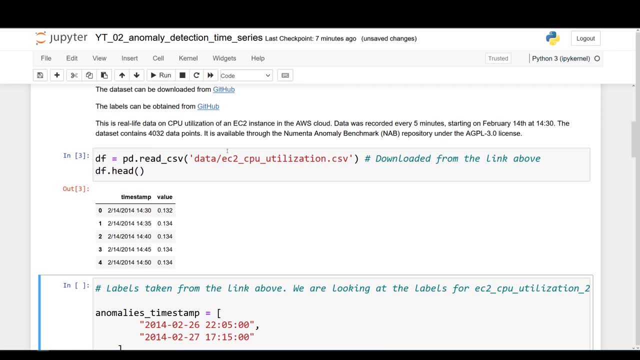 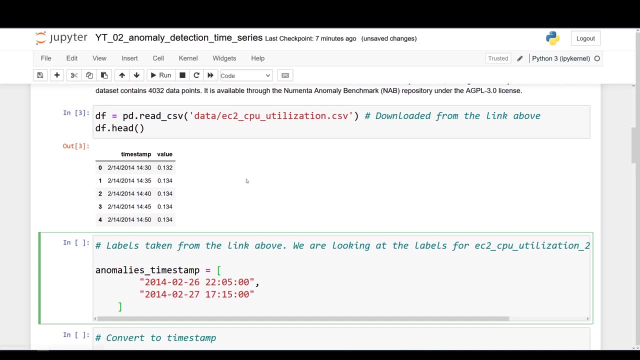 try things with different data sets after this video. so let's go ahead and read the data. so, again, this is the, the data that i downloaded from the link that you can find here, and then, once this is done, we're also going to take the labels. so the labels- this is the second link that you can see here. so, basically, here in our data set. 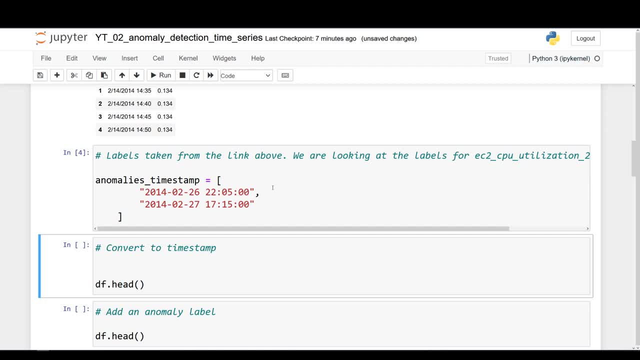 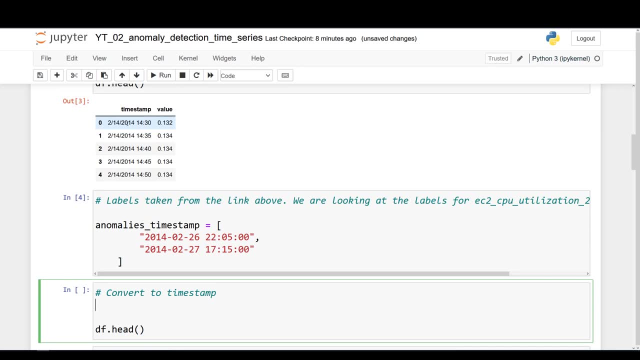 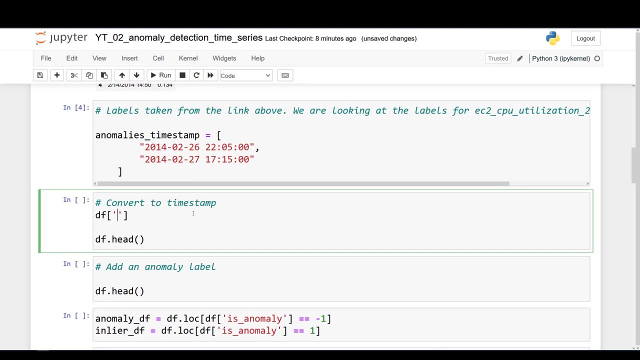 we only have two points that are anomalies in this case. so before we move on, as you can see here on the timestamp, we don't have an actual timestamp type, right, because of those slashes- let's actually convert those dates to timestamp. so i will say that df timestamp is equal to pd dot two date time. 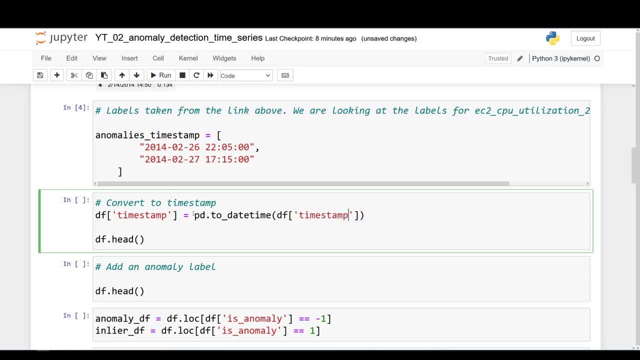 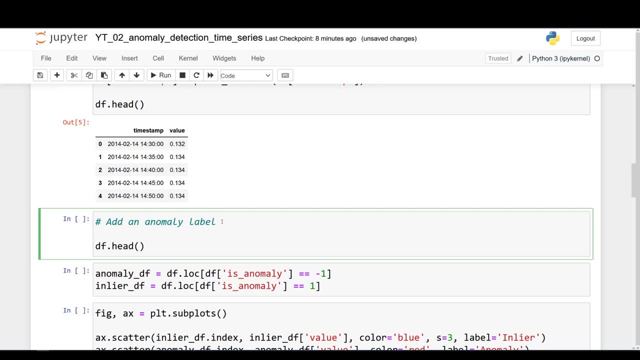 and then pass in again the timestamp column. perfect, and now we have the right format. so this is great. we can actually move on. um, and now i am. what i'm going to do is add an anomaly label. so you know, we are trying to do anomaly detection, so of course we need to find a way. 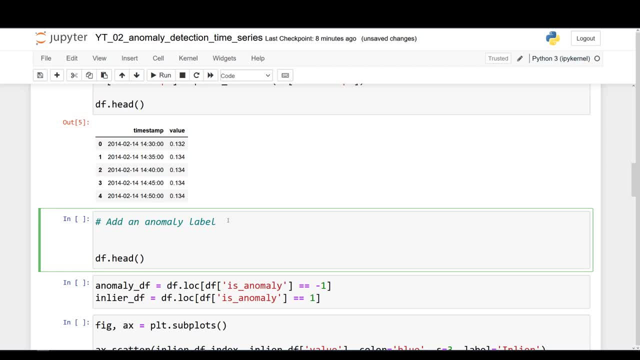 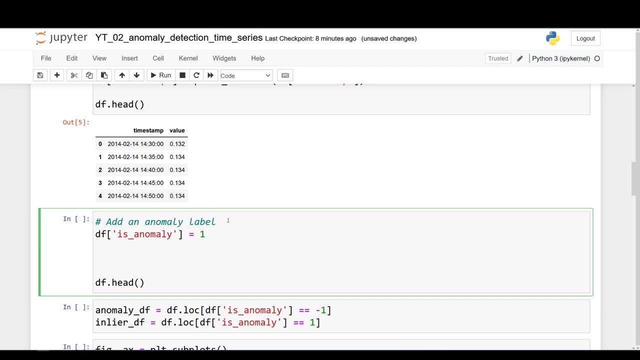 is our method correctly identifying the anomalies or not? so, and for that we need an able label. so df is anomaly, so this is a new column that i am creating is going to be equal to one, so i'm going to add an anomaly label. so by default, one here in this case will mean inliers, so not an anomaly. 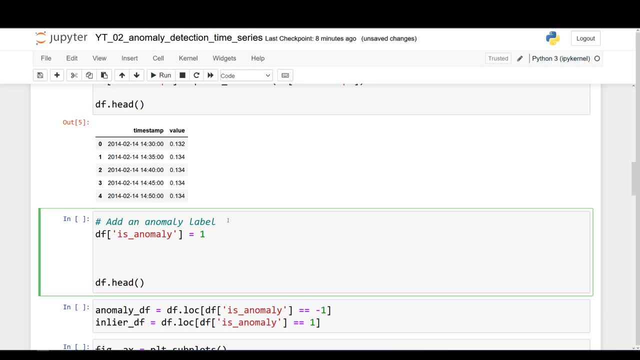 minus one will be an anomaly. this is basically the standard that scikit-learn is using as well. so all the models you know, a normal point will be one and an outlier will be minus one. so we are using the same thing here just to keep everything easy later on when we start modeling. 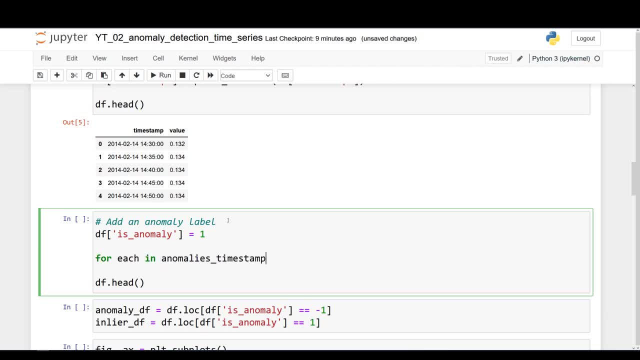 so for each in anomalies timestamp. so now i am going to identify my anomalies. i will say that df lock and then here df timestamp, where it is equal to each. then you will say: that is anomaly is going to be equal to minus one perfect. once this is done, we can go ahead and display the head. so now, as you can see, we have our timestamp. 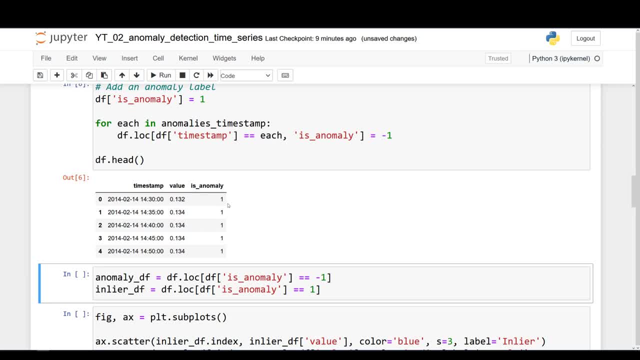 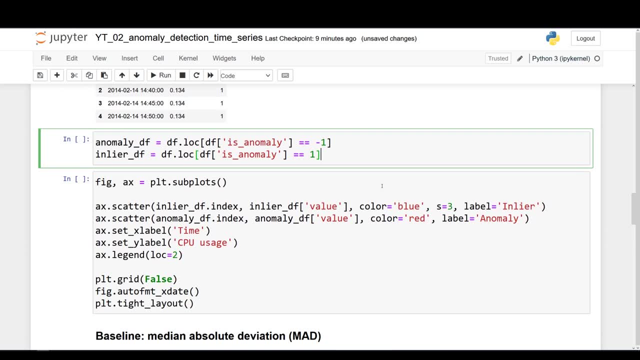 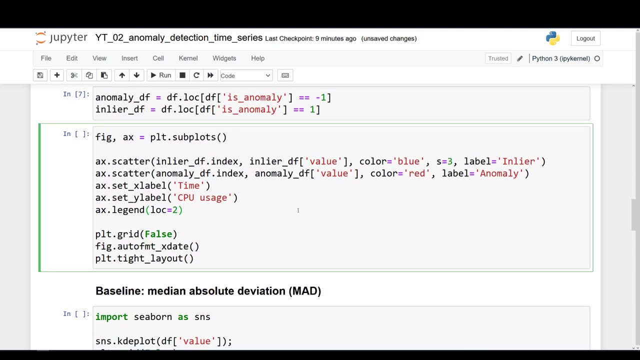 we have the value, and now we have this label in the is anomaly column telling us if the point is an inlier or a outlier. and now let's quickly visualize our data. so here i'm just separating my anomaly and inlier data and then i am making a plot, very standard plotting code here and you should get. 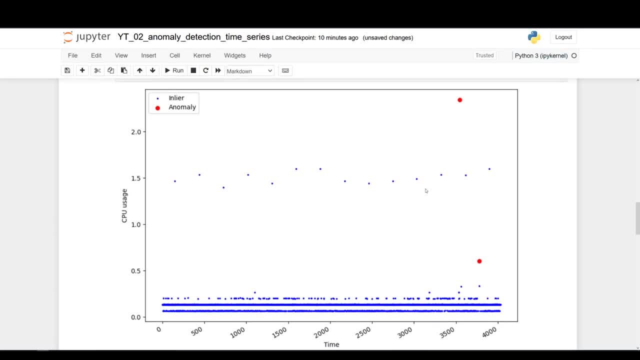 the following. so let me zoom out a little bit so you can see everything perfect. so now, as you can see, we have our data. so in blue, this is all the normal points, so the inliers, and in red the outliers. so, as expected, right, just like we have seen in the slides, the two red dots are: 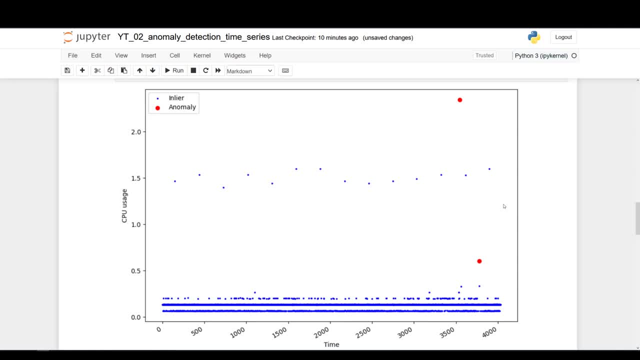 anomalies, and those are the points that we are trying to find out now, of course, keep in mind, right, because it is anomaly detection, we are detecting very rare events, which is why we only have two points here, right. so it's going to be very hard for our model, you know, to find those. 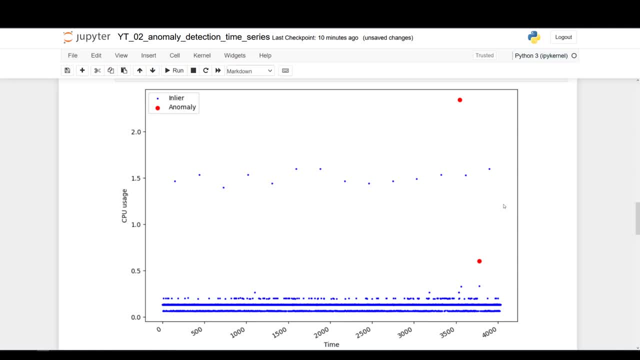 points and also when we evaluate it. it's really like either you hit or miss right. so either you find uh this, these one or two points, or you completely miss them right. so it's going to be a pretty interesting, pretty hard as well. uh, also notice that we have a lot of constant values. 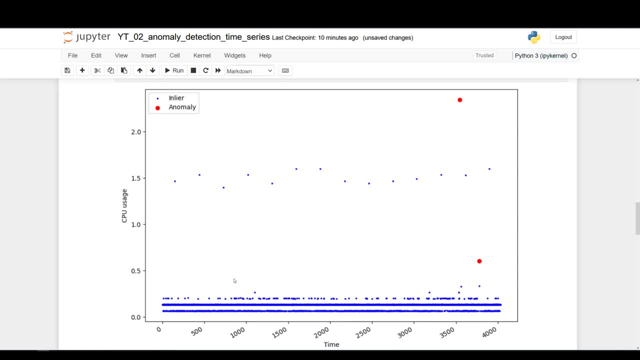 right. so we have all those flat lines here at the bottom in blue, which is uh, which is interesting, right. so we'll see how, uh different algorithms take that into account. so, uh, that's really it for this uh little part here. let's go back into the slides so that we can learn about our very 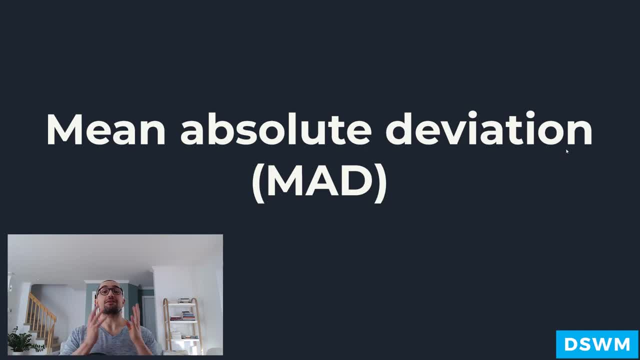 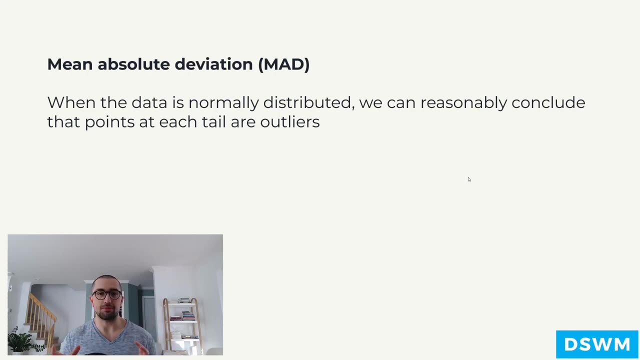 first method. all right, so we are back and let's take a look at the very first method that we will use here to identify outliers in time series data, which is the mean absolute deviation or the mad. so the mat is fairly intuitive and i would say this is some kind of a of a baseline method. okay, so it. 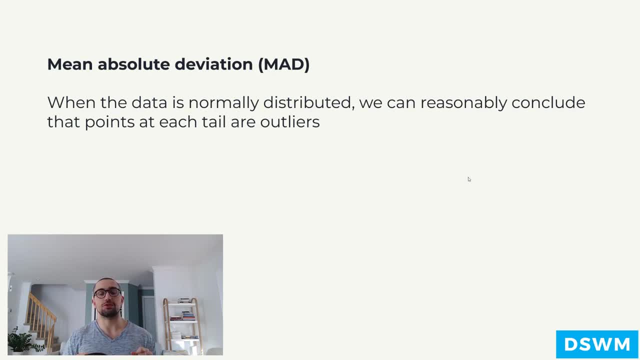 will work, but not all of the time, because we really have to use it in very particular situations. okay, so the idea behind the mat is that when your data is normally distributed right, you can reasonably say that points at each tail, at each end of the tails right, are outliers. okay, that? 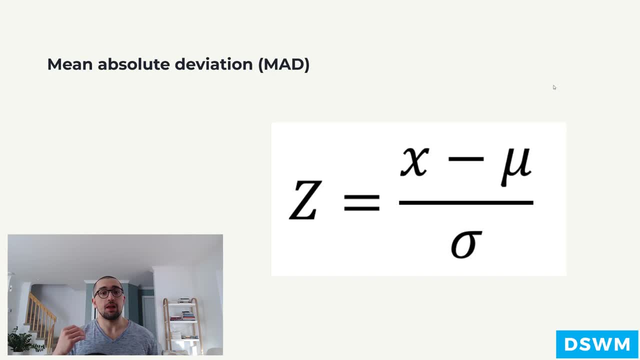 makes sense. so, for example, if you take a and this is done, um, by using these methods, uh, for example, we can go ahead and show it using the z score method, right? so if your z score here, you can see this is basically the point minus the means divided by the standard. 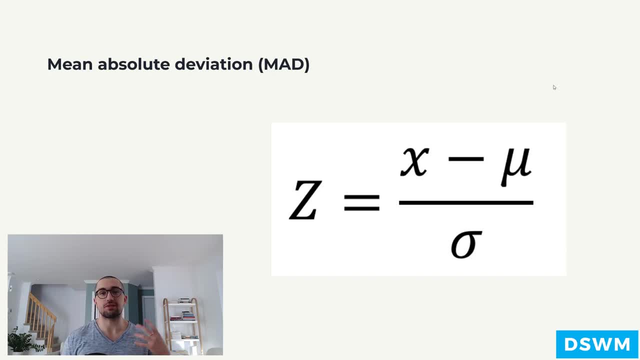 deviation. and so this is how you can say: is my point an outlier or not? so usually when your z score is above like three or 3.5, usually we conclude that it is an outlier. so this is basically what we are visualizing here. right here we can see this normal distribution and then on the x-axis, you have the z-score. so as you can see, here i set a threshold of three. so anything you know above three or below a0, fravi, these are three points. so in a lot of cases where this map can take ways between Jack's x and it will fall through several��c demand and so on can make the foundation six for umas. 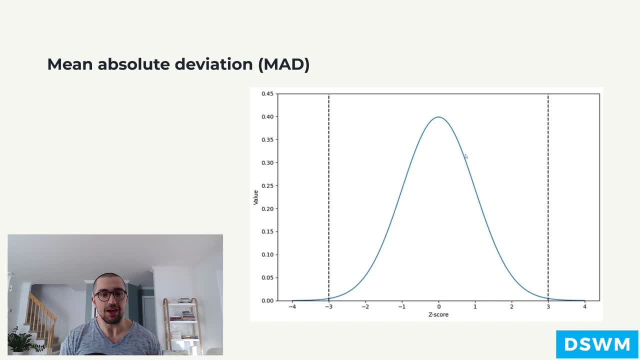 3 or below minus 3, you could say that those are outliers. Now, because you have outliers in your data, they will affect the mean And because you are using the mean when computing your z-score, you are affecting the z-score. 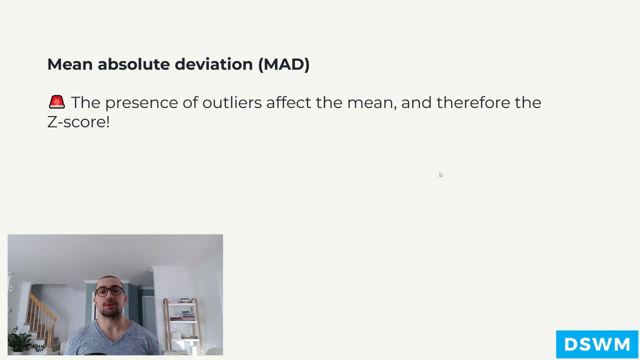 as well. So we need to find something more robust, something that will not be impacted by the presence of those outliers, Which brings us to the robust z-score method, That, instead of using the mean when computing the z-score, instead we are going to use the median, Which we know is a statistic that. 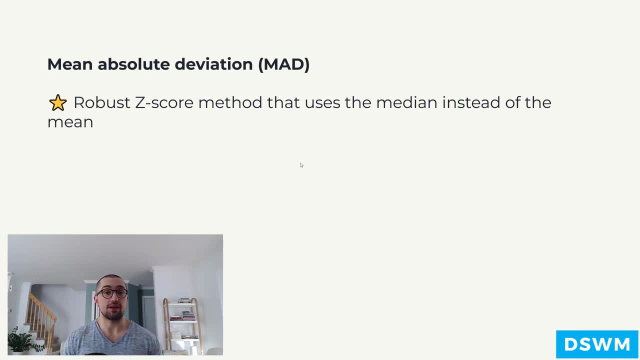 is much more robust and stable when we when we have the presence of outliers. So the MAT basically is this formula, as you see here. So it is basically the median of: Basically it's the absolute difference between the values of sample and the median of the sample. And then the way we calculate the z-score is doing in this. 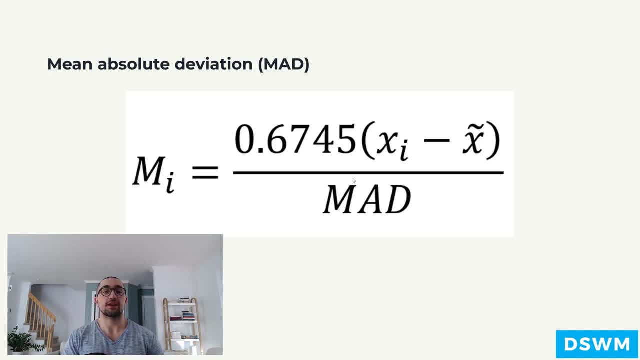 following formula: So 0.6745 times the value minus the median of the sample divided by the math. And by the way, you might be wondering why do we need to scale by 0.6745.. This is because the z-score uses the median absolute value. It's always smaller than the standard deviation. 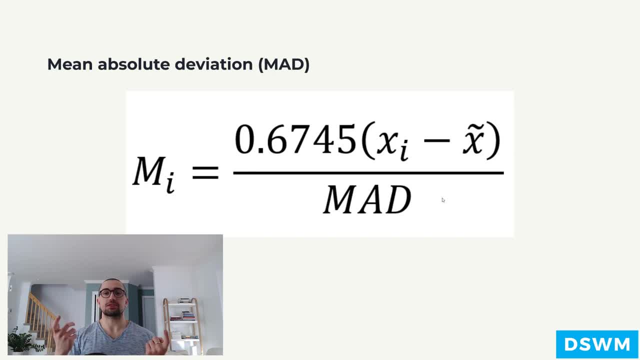 basically. And so to bring it back to something that looks like a z-score, so because you're dividing by a smaller number, your number is going to be a bit larger. So to bring it back to the scale of a z-score, you multiply by 0.6745, which usually brings it. 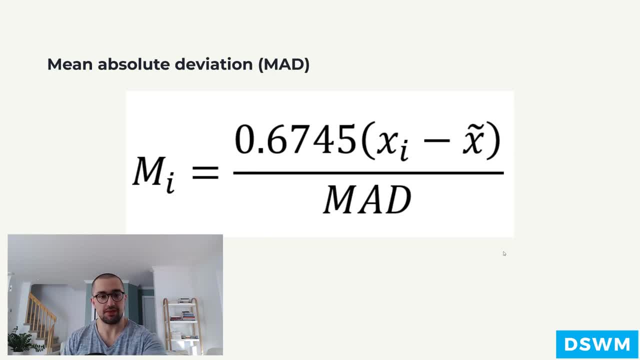 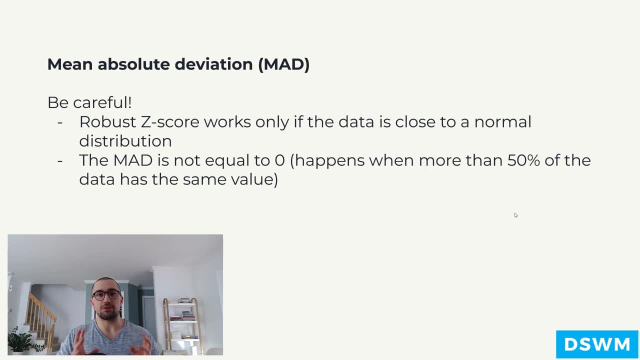 back to the scale of a z-score And so you can use it as a z-score method. Now you have to be careful. So, like I said, this is like some kind of a baseline method, very naive. You have to be careful. The z-score method only works if your data is close to a normal distribution. 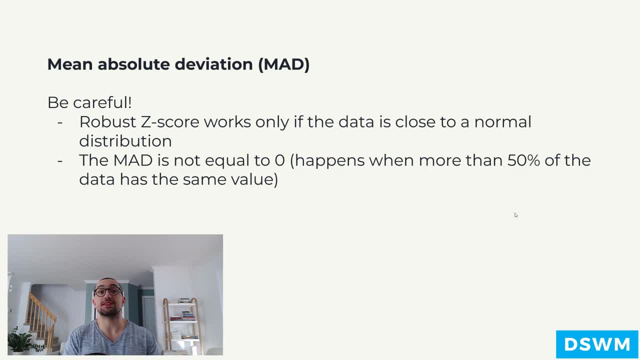 so, first of all, And second, if your math is not equal to 0. So, of course, if you're dividing by 0, it's going to be very bad, And that happens usually when more than 50% of the data has the 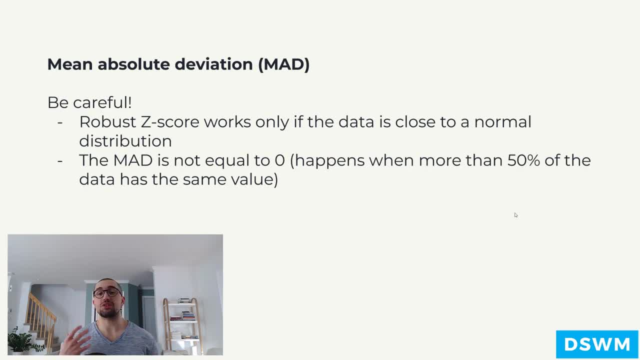 same value. So if that is the case, usually you cannot use the math in that situation. Now, of course, you might remember, our data has a lot of constant values, a lot of flat lines, And so here, in this case, 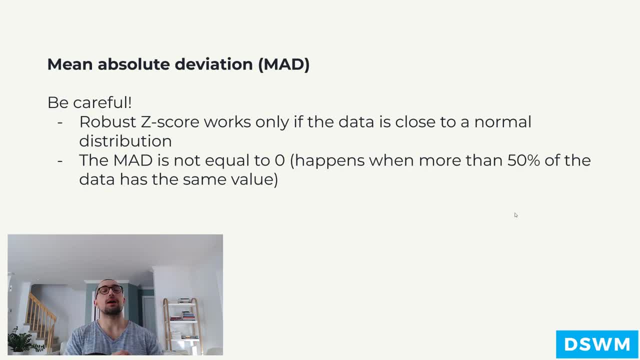 implementing the math is definitely not the best of ideas, So I am expecting this not to work very well, but we're still going to implement it, just so that you know how to do it if you ever encounter that kind of situation. So that's it for this. Now let's go back into the code and implement this. 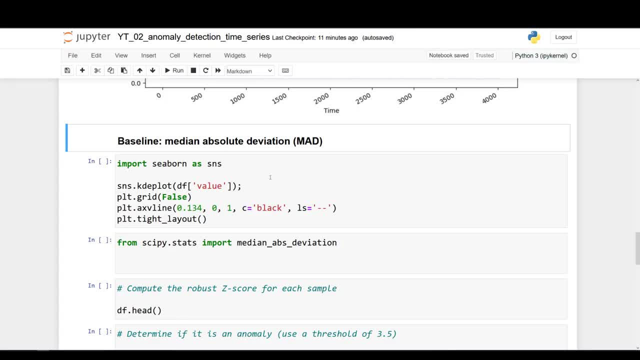 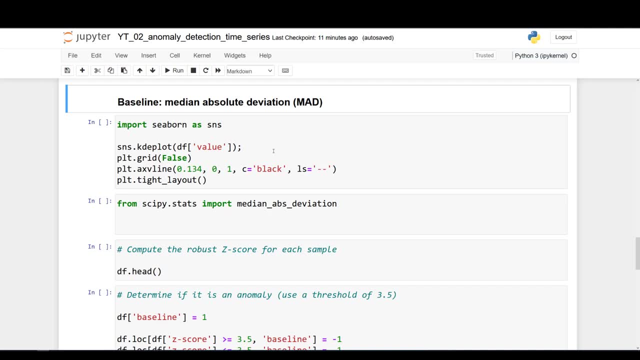 robust z-score method. Okay, And we are back into the code. So I'm just resuming the same notebook that we have started before, And now let's actually implement our kind of a baseline method here, which is the medium absolute deviation or the MAD, And so for that, as you, 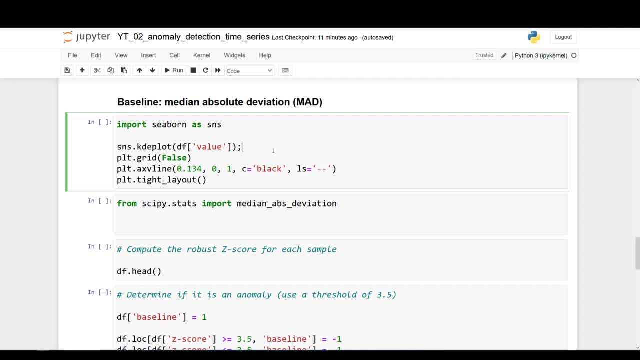 remember the MAD can be used in two situations right, When your data is close to a normal distribution and when your MAD is not equal to 0, meaning that more than 50% of your data is actually equal to the median. So for that we need to take a look at the distribution of our 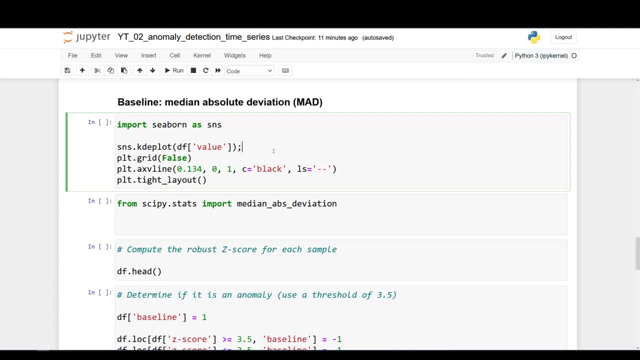 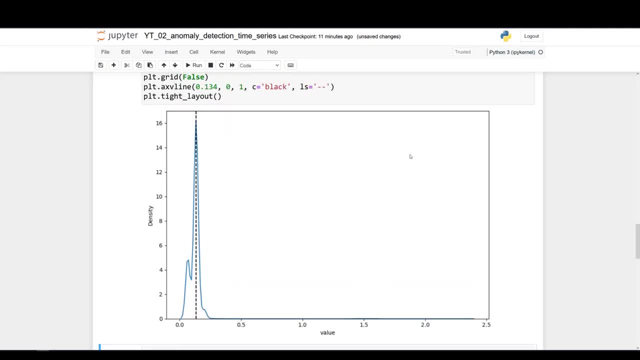 data, see if it makes sense in this case. So here again, just to clarify: we are using the same again, just plotting the distribution of my data, very standard, And we get the following: So this is very problematic, right? So, as you can see here, this horizontal line indicates the 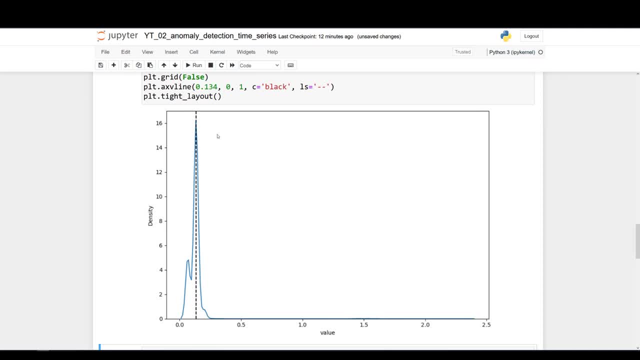 median. and then we also: it matches the peak right. So that means that a lot, a lot of the data actually falls right on the median. okay, So already first red flag. okay, I don't know if it's actually 50% of the data that falls on the median, but a big proportion of it actually falls. 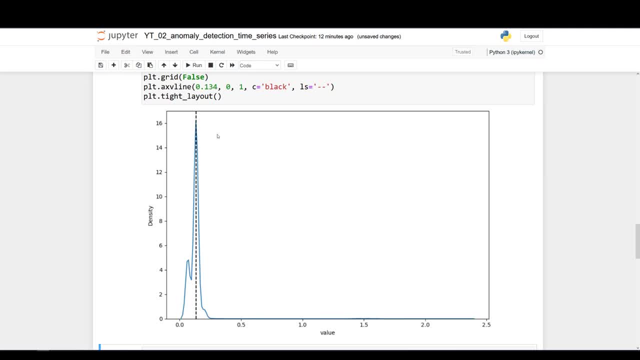 on the median. So already the MAD probably is not going to work very well. And also, looking at the distribution right, This is definitely not a normal distribution. It's very skewered to the left. So again two red flags, in this case right: It's not a normal distribution and a big portion. 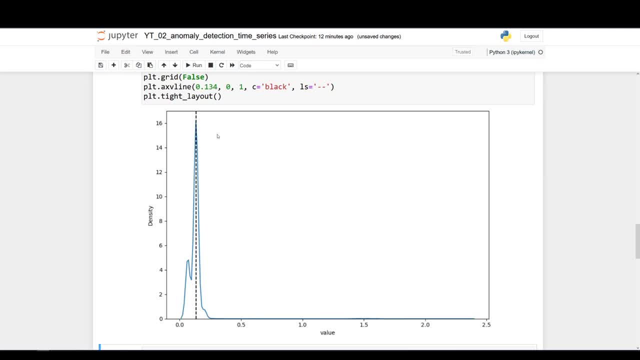 of the data actually falls right on the median. So I'm really expecting the MAD not to work here very well, but that's okay. I still want to implement it For you guys so that you know how to do it. So if you ever encountered this kind of situation, 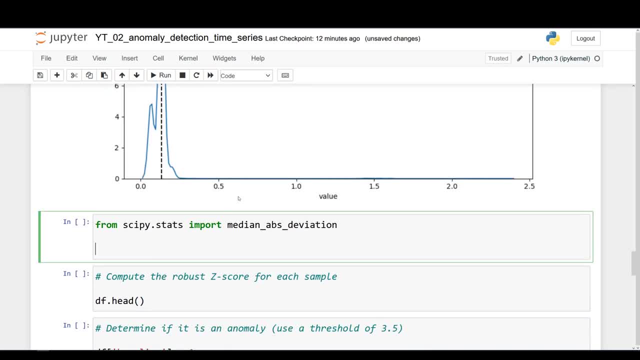 you'll be able to do it okay. So, with all that in mind, let's actually implement this mean absolute deviation, or like the robust z-score method actually. So, actually, the median absolute deviation can be imported from SciPy. So this is what I'm doing here. 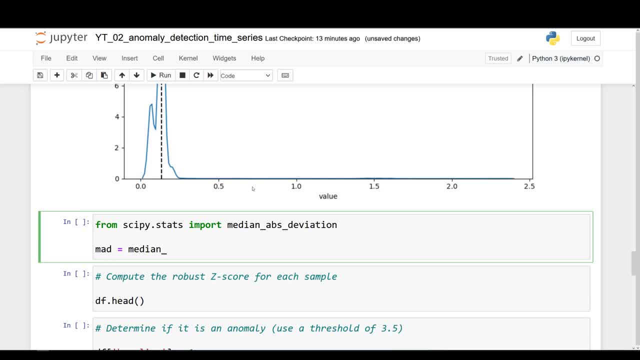 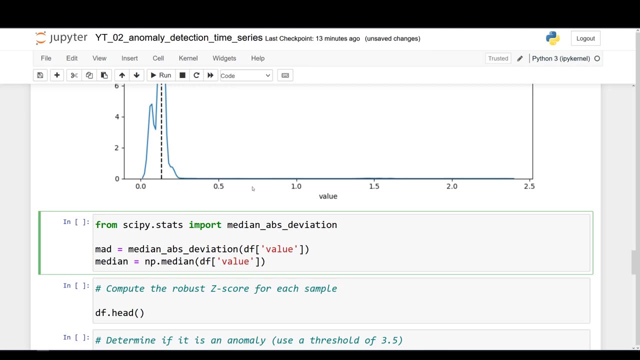 So here the actual MAD, it's median abs deviation. So it's actually computed here of the df value, perfect. and let's also take a look at the median. so the median is np, median df value. so we are going to need those values right later on to compute the, the robust z score. and then once 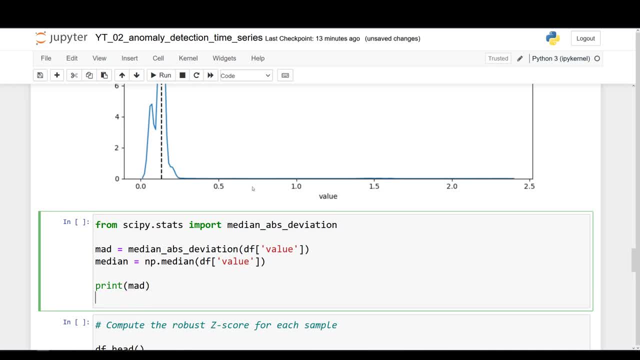 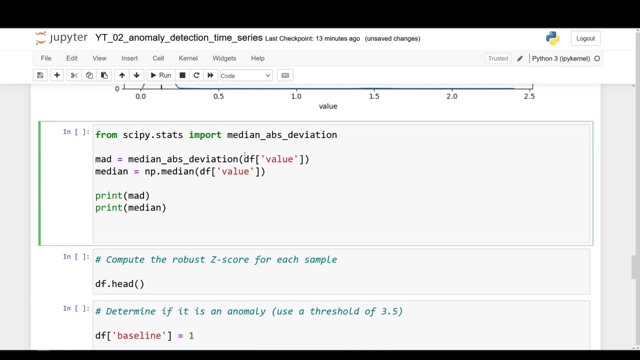 this is done, we can actually print them. so why not? let's print the mad and let's print the median, like so, and then let's actually define our function already to compute this robust z score. so i'm just going to follow the formula that we saw on the slide. so compute robust z score. we. 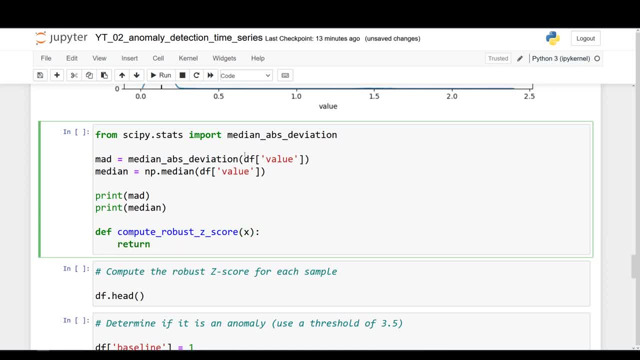 pass in some value and this will simply return 0.6745 times x minus the median and everything divided by the bad. so this is simply the formula that we saw to compute the robust z score. so let's go ahead and run this cell and you should get the following: so: 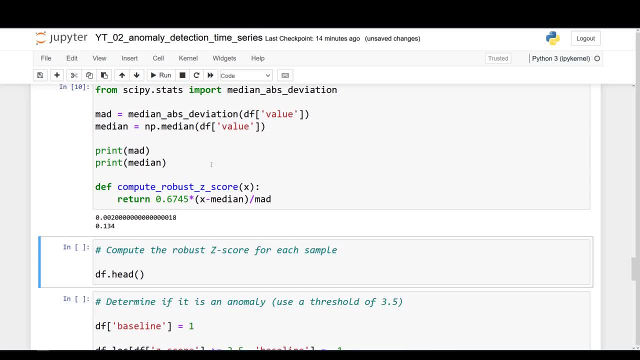 i, as you can see, big problems, right, our mad, our mean, our median- sorry, absolute deviation is equal to 0.002. so it's not exactly zero, right, um, but it is very close to zero. so what's going to happen now? probably is that because your mad is so small. basically any, 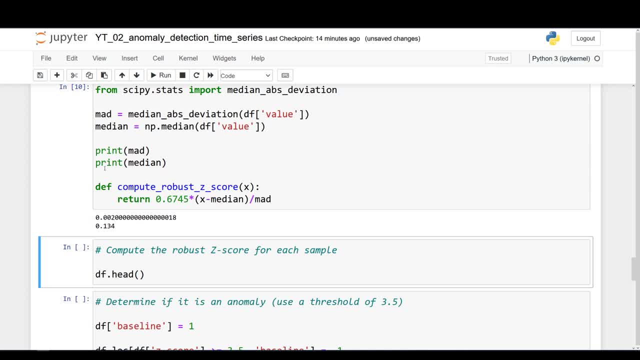 point that is slightly off from the median right. so anything slightly over or slightly under the median will probably going to get flagged as an outlier, because, keep in mind, you're dividing by the mad and so here you're dividing by 0.002, which is a very small number. so your z? 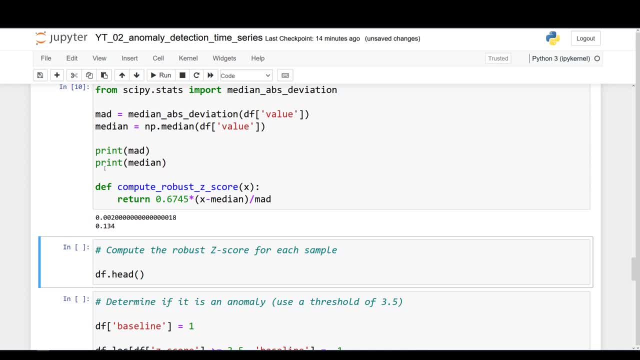 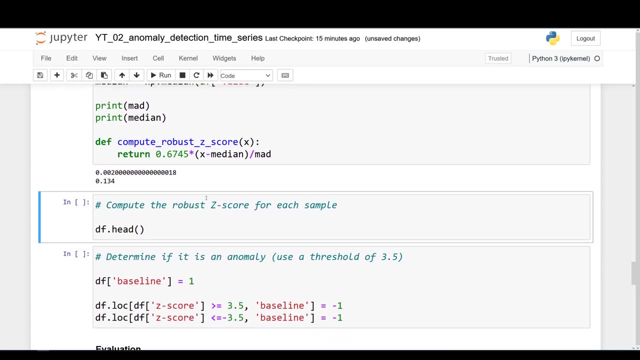 score is going to be very large, right and so even setting a threshold to like 3 or 3.5, you know, chances are that your z score is going to be so large that again, any value somewhat off from the median is going to be flagged as a outlier. but still, you know, let's keep moving ahead. just to: 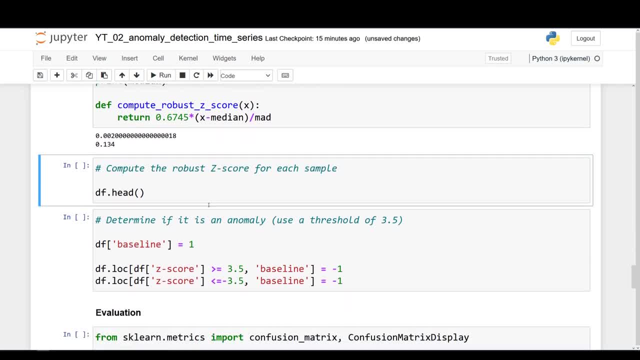 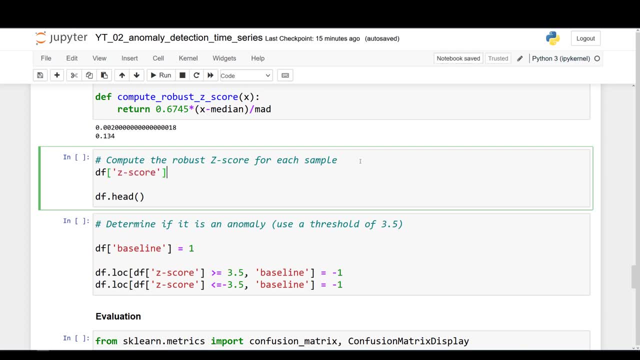 just so you can know, you know how to apply this method. so let's actually compute the z score for all of our samples. so i will say that df z score is going to be equal to df value, and then we are going to use the apply method here, which is compute robust z score, just like so. so let's go. 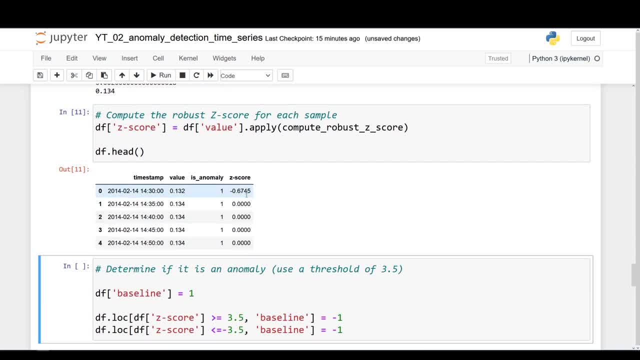 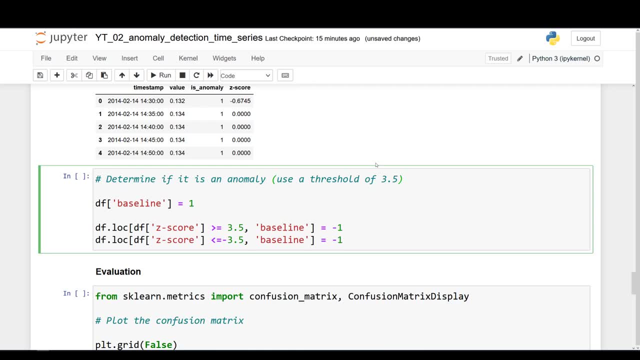 ahead and display the head now, as you can see, for each of our sample. now we have our z score perfect, and then, depending on the z score, we can now determine if a value is either an outlier or an inlier right. so this is what i am doing here. so, as a baseline, you know everything is going to be. 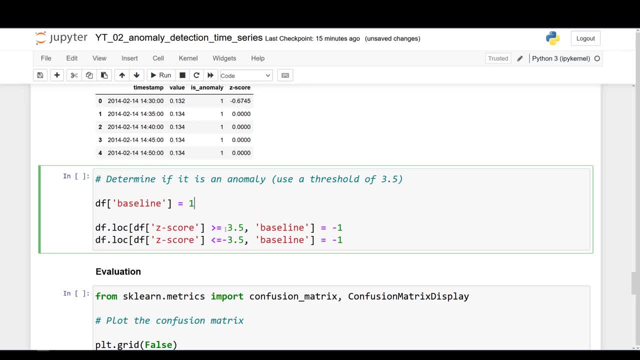 an inlier, and then i use a threshold of 3.5. so here if the z score is greater or smaller than so, if it's greater than 3.5, you know it's an outlier, and if it's smaller than minus 3.5, you. 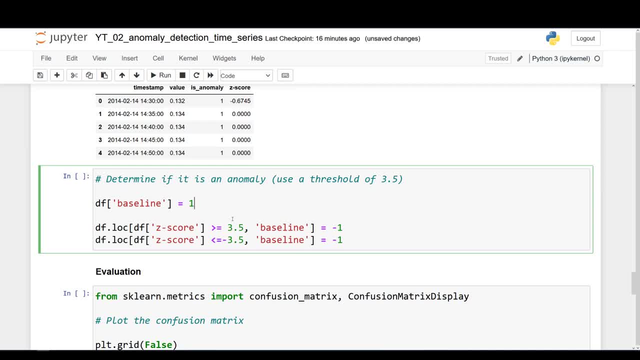 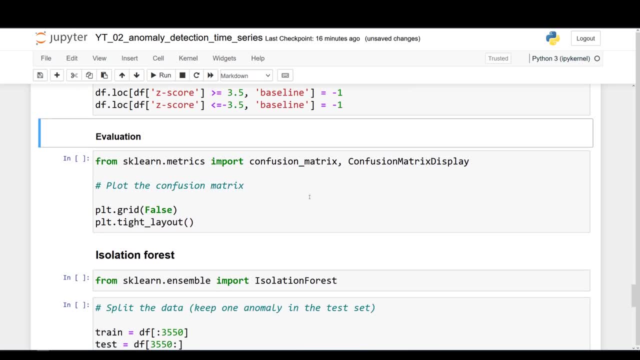 know, just to make sure that you cover both ends of your distribution, then it will also be an outlier. so minus one. so let's run this perfect, and now we can move on to the evaluation. so how are we going to evaluate our model? very simple, we'll use the confusion matrix. okay, so 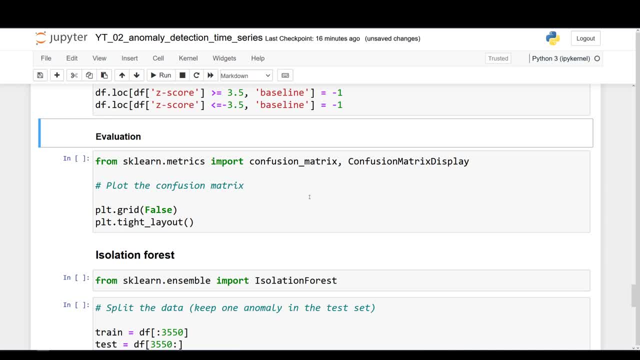 you know. so we can see what were the predictions from the model and see if the right label was assigned to the value. so very simple: you can import the confusion matrix and confusion matrix display from scikit-learn and then it's just a matter of plotting it. so i will say that cm. 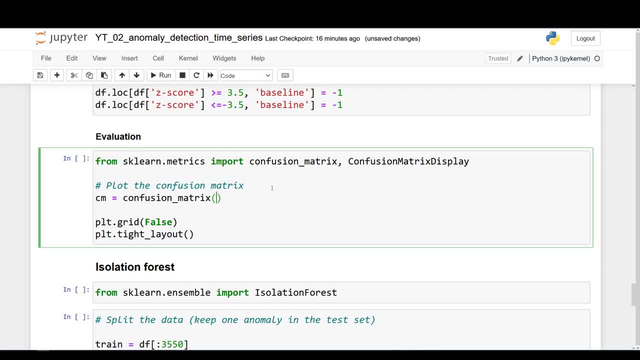 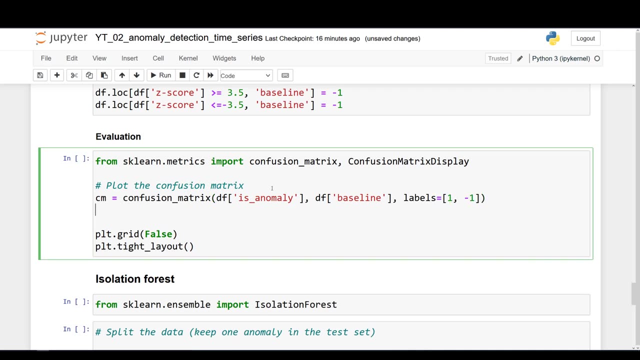 is equal to the z score, and then we can see that the z score is greater than minus 3.5. so we can use the confusion matrix. and then you pass it- df is anomaly, like so- and then you also pass it. the baseline column perfect and the labels in this case is going to be one and minus one, all right. 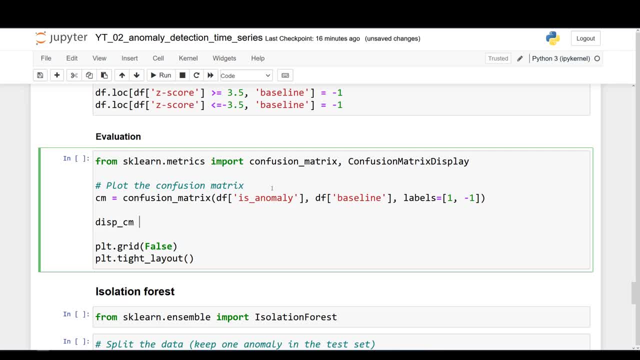 and then you say that this cm, so display, the confusion matrix is going to be a confusion, oops, confusion matrix display, like. so passing your confusion matrix and then again display labels is going to be equal to 1 and minus 1, all right. and then you can simply say this: cm dot plot. 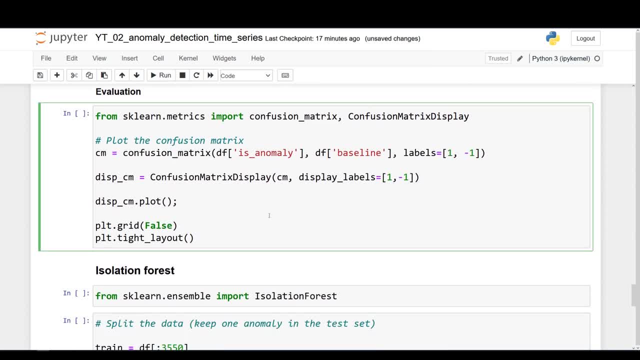 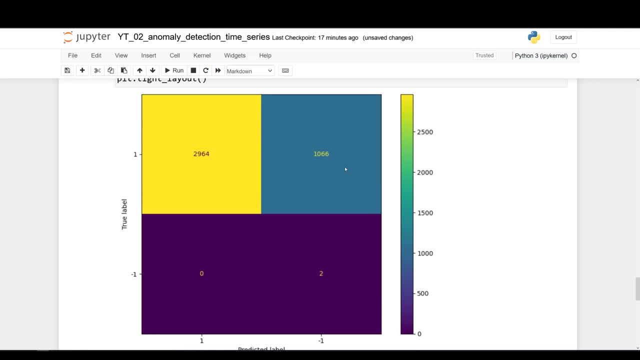 like so semicolon at the end and let's go ahead and run this and you should get the following. so again, let me zoom out just a little bit: uh, and so this is what you get. so definitely, uh, it was pretty bad. right, it is fairly bad. so, of course, as you can see, it, did uh correctly label the two. 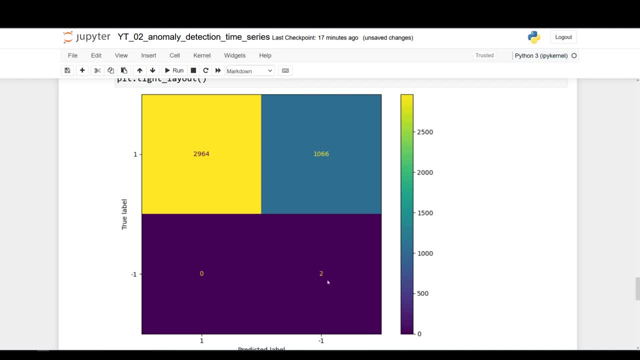 outliers that we had earlier. so we can see that it did correctly label the two outliers that we had in our data, right? so this is what you see: this number on the bottom right corner. so this is great, right, the two outliers that were actually outliers were identified by this. 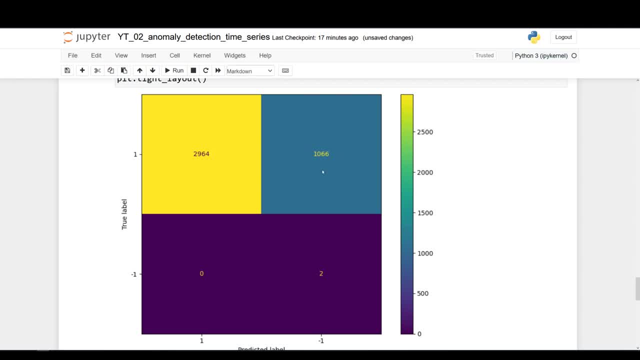 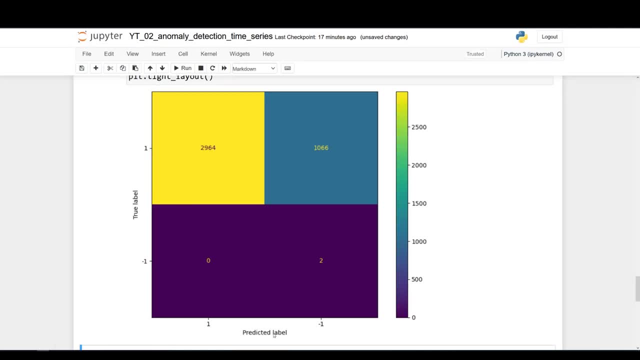 robust z score method. however, you can also see that a lot of data was flagged as an outlier when in fact it is not right, so uh. so let me zoom out again. predicted label minus one here, but the true label is equal to one. so that means that the model incorrectly labeled normal data as an. 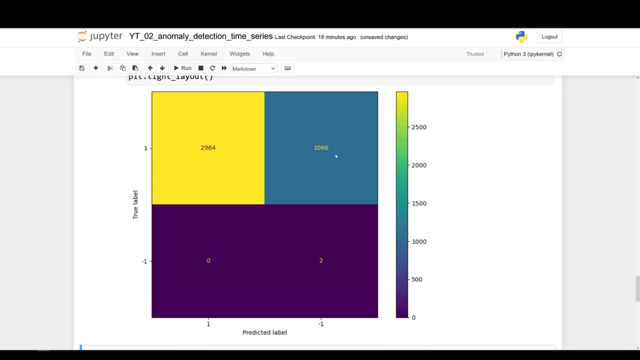 outlier, and so, again, this is to be expected. so we can see that the model incorrectly labeled normal data as an outlier, when in fact it is not right. so this is to be expected, right, we had a lot of flat values here. in this case, the math was very close to zero, so again we see actually what is. 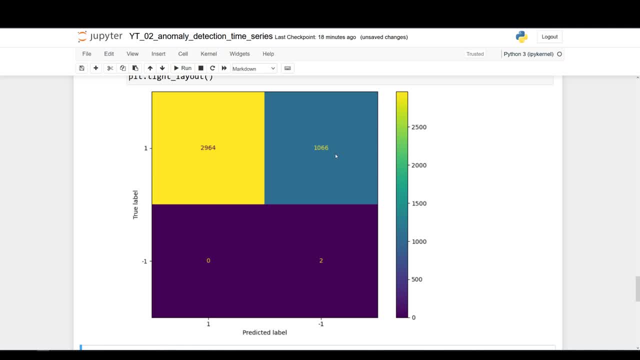 happening. right, anything that slightly deviated from the median uh was flagged as an outlier because of this method. okay, but again, it doesn't really make sense to use it here, because not a normal distribution. that was very close to zero, but now you actually know how to implement this. 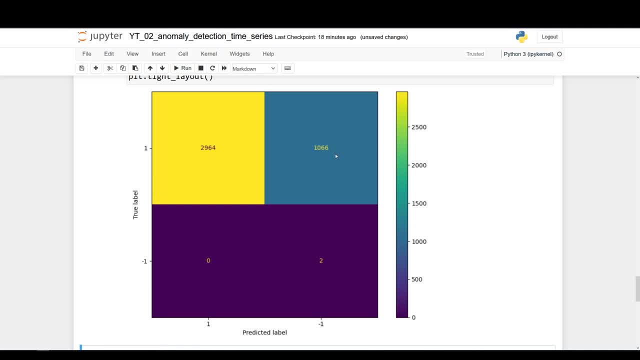 method. so if you ever encounter that kind of situation, right, you know how to implement this baseline method and, uh, you can see that the method is very similar to the one that we used in the first case so far. uh, who knows, maybe it's gonna work better in some other scenarios, but anyway, 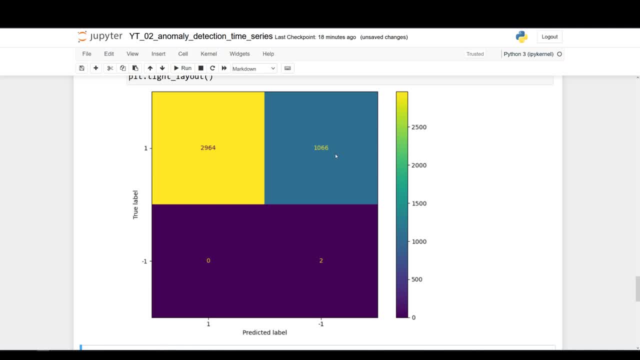 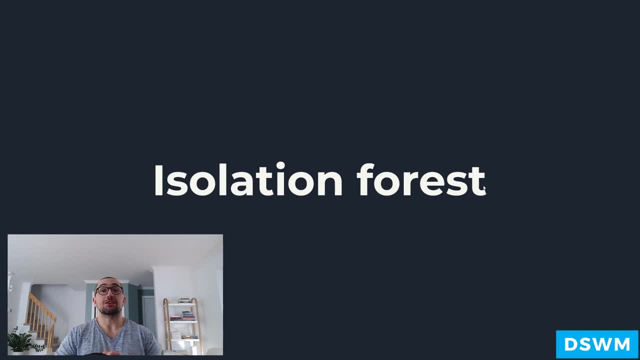 that's it for the math, for the robust z-score method. so let's go back into the slide. we'll learn about the isolation forest and then we'll come back into the code to implement it in python. all right, and now let's take a look at the isolation forest algorithm. so no surprise. 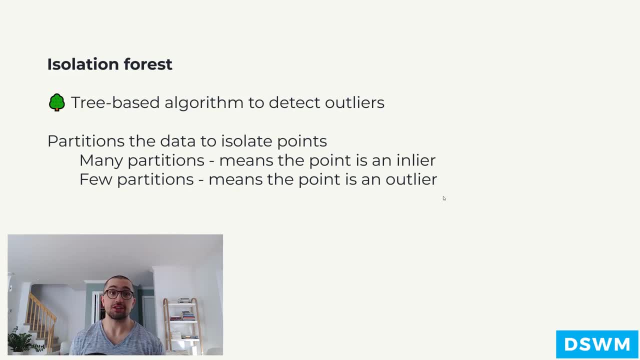 here. this is a tree based algorithm that is often used for anomaly detection, and basically the algorithm starts by randomly selecting an attribute and then you randomly pick a random, selecting a split value between the maximum and minimum values for that attribute, And so the partitioning is done many times until the algorithm has. 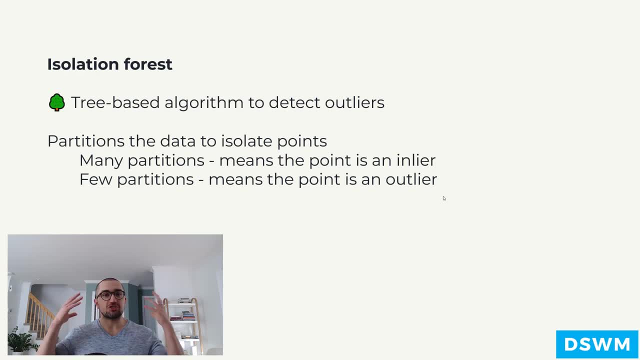 isolated each point in the data set, And so the general idea behind this is that if it needs many partitions to isolate that particular point, then it means that the point is an inlier. However, if you require few partitions to isolate it, then it means that the point is an outlier, And this really makes sense with 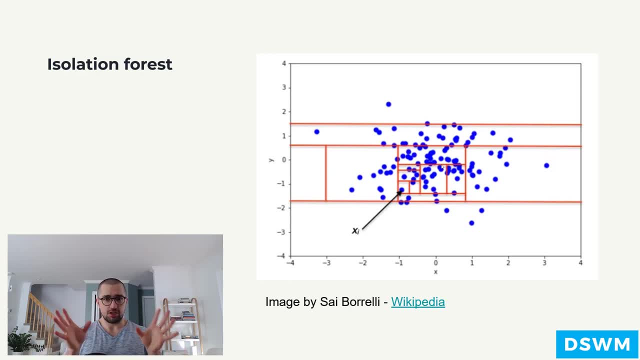 this picture here. So, as you can see, every red line, so a tree right. It can only make either horizontal or vertical lines, So every line is a partition here, And so to isolate this blue point here, that is with the arrow here, XI to 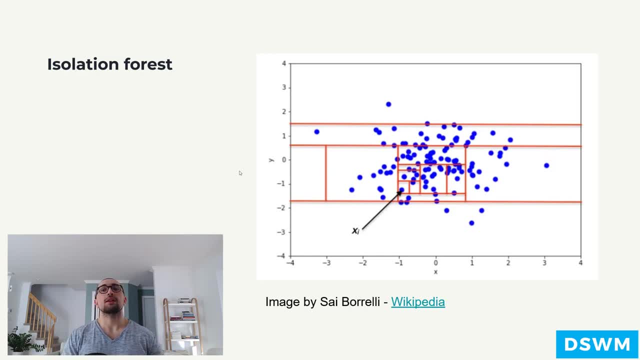 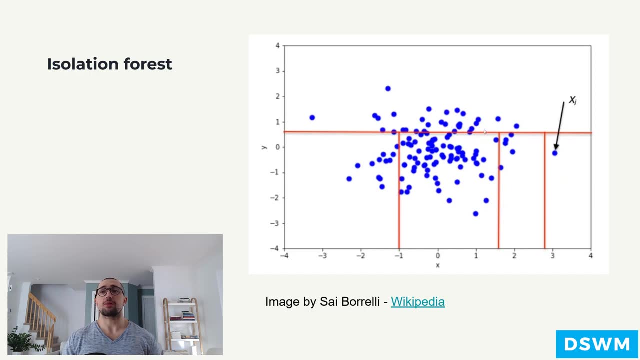 isolate it. as you can see, it required a lot of partitions, right? So this means that this data, well, is likely to be an inlier. It's a normal point, okay, However, and when you take a look at this point here, XJ now, in this case, in only. 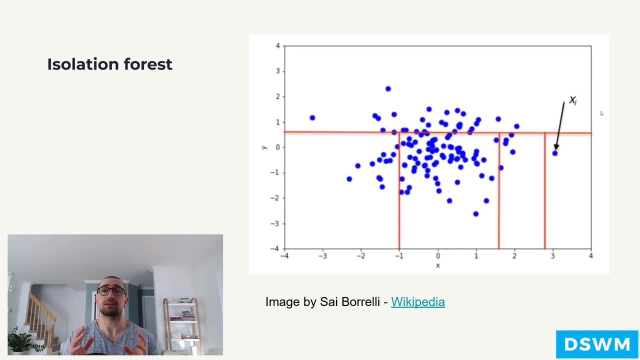 one case. it's a normal point. So if you take a look at this point here XJ and you take a look at this point here XJ, now, in this case, in only one case, it required four partitions to isolate it right completely. So in this case, 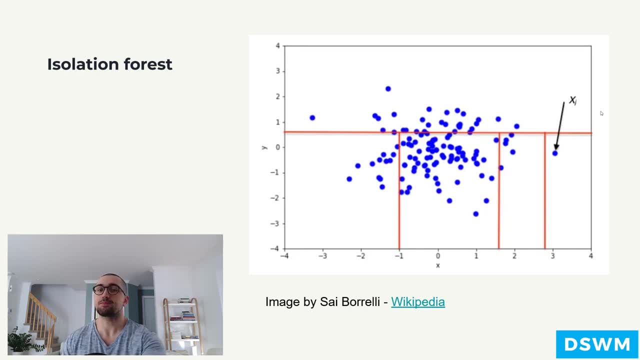 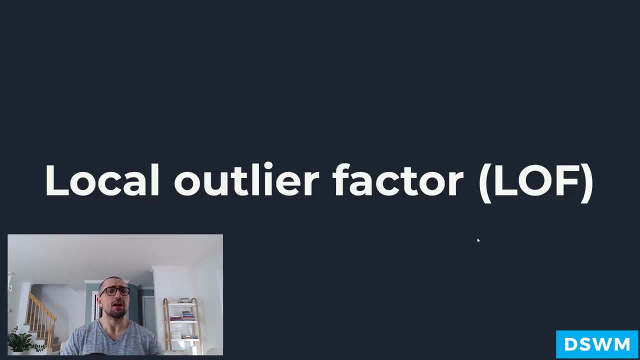 this point, XJ is likely to be an outlier because, well, in this case you know, very few partitions were necessary in order to isolate it completely from the rest. So that is really all there is to it about isolation forest As you can. 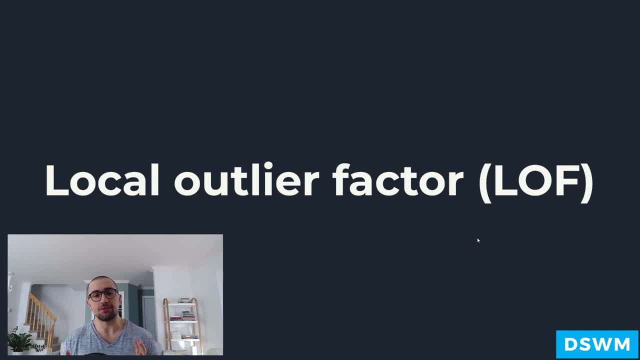 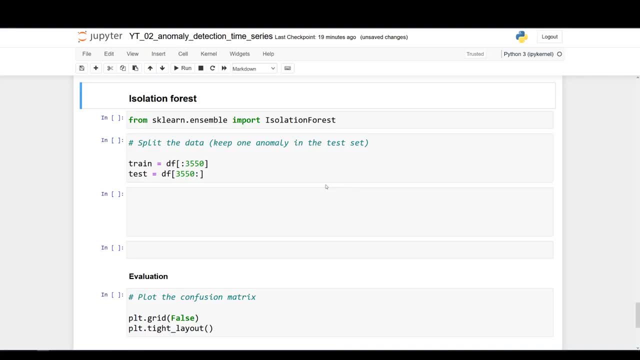 see, very simple, very intuitive. So let's implement it right now in Python, and then we will come back to take a look at the last method, which is the local outlier factor. Okay, and we are back, and now let's implement the isolation forest algorithm. 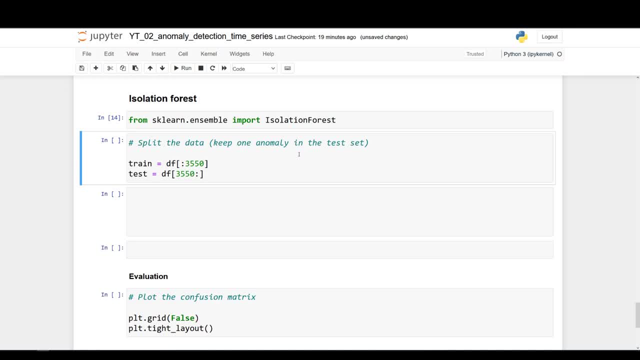 So very simple. we're going to import it from scikit-learn, And here I would like to do something a little bit different. So instead of looking at all the data and seeing if the model can actually identify if it is an anomaly or not, let's consider the scenario. 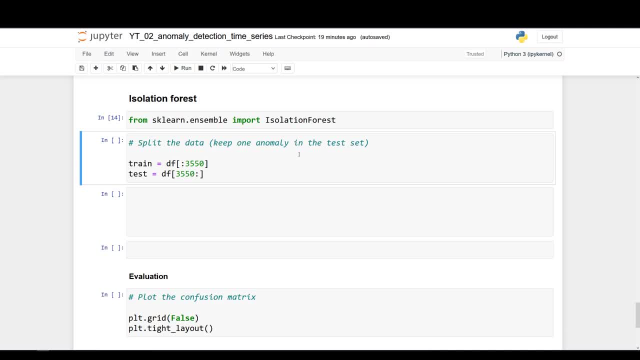 where you have data and then you want to see if a future point or if a new data point will is an anomaly or not, right? So this is really when things get interesting, right? You don't want to know if something in the past was necessarily an anomaly, but 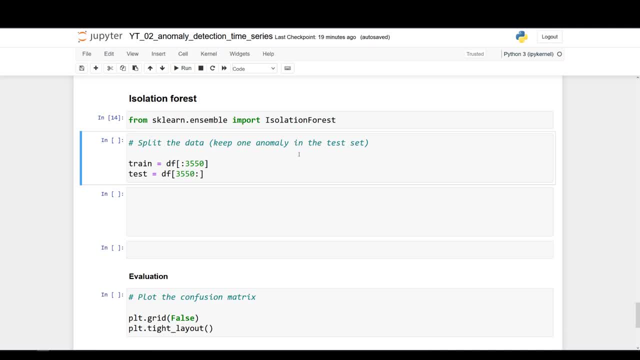 it would be interesting to know if a new data point coming in, is this one an anomaly or not? So this is what we are doing here. so this is why we are splitting the data like so, in such a way that we have one anomaly point in the training set and then one anomaly. 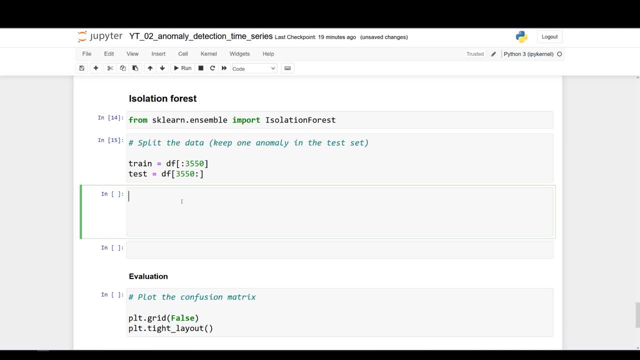 in the test set. So here we'll evaluate the model in its capacity to identify this new anomalous point in the test set. So to use those algorithms you have to start with an. you actually need to set a contamination level, So the contamination is really just the number. 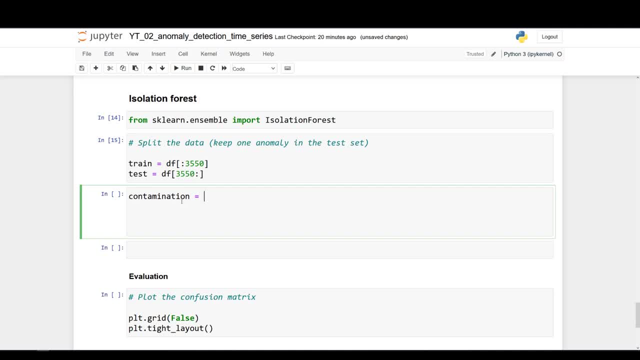 of anomalous points in your training data. So in this case it's one over the length of training. So this is something that I know. I did split the data just so that we have one anomaly in the training set, one anomaly in the test set. So the contamination is simply one divided by the entire. 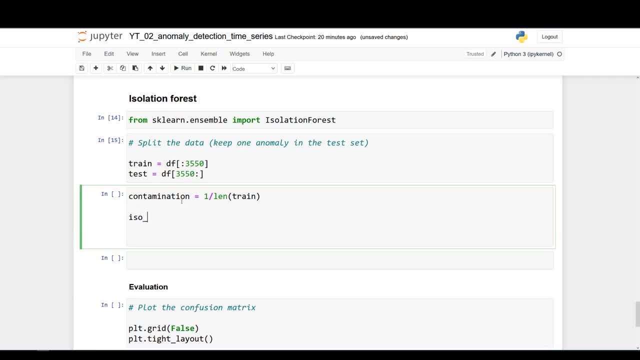 number of samples in the training set, And then, once this is done, we can go ahead and initialize our model. So isoforest is isolation forest like, so The contamination is going to be equal to contamination. And then here let's specify a random state. In this case I will set. 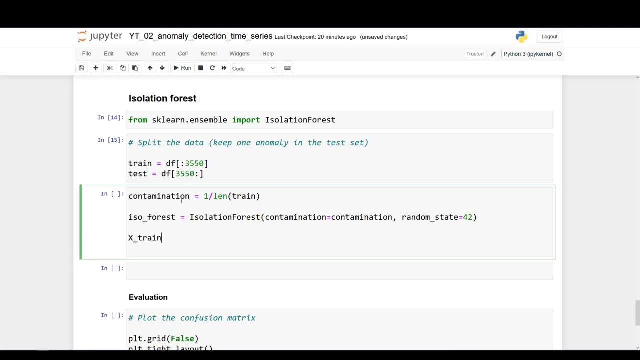 it to 42.. All right, And then x-train has to be reshaped, So x-train is going to be equal to train values, and then dot values, dot reshape minus one one so that we can feed it to the model. And then it's just a matter of fitting the model So isoforestfit, and then you pass it. 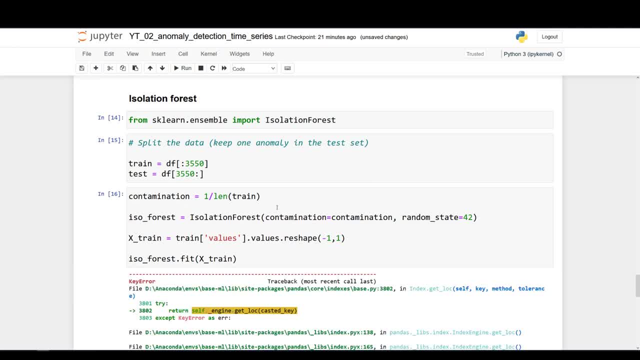 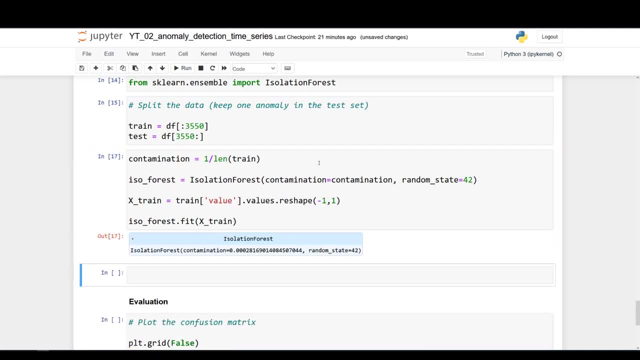 x-train, Perfect. So let's run this, and it shouldn't take too long to fit. And I made a little mistake here. The column is not called values. The column is called value- All right, Perfect. So now that this mistake is fixed, let's go ahead and run this. So let's run this. So let's run this. So let's. 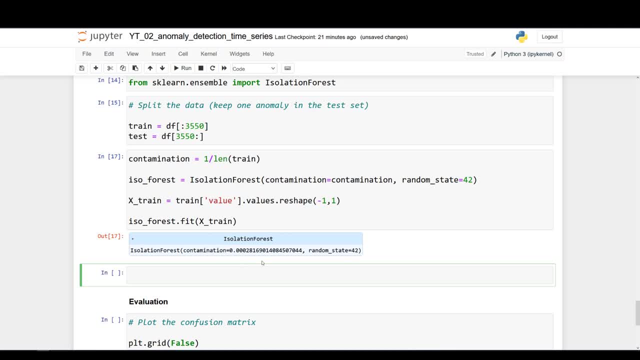 fix it Perfect. Everything worked correctly. And now that the model is fit, we can go ahead and make some predictions. So Preds is going to be sorry. So, Preds, isoforest is going to be equal to isoforest dot. predict and then pass in your test data, which also has to be reshaped, So test. 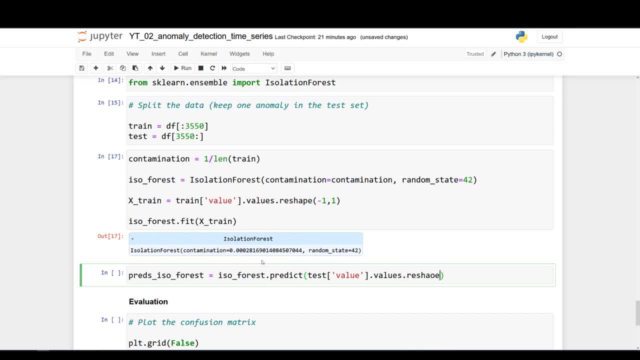 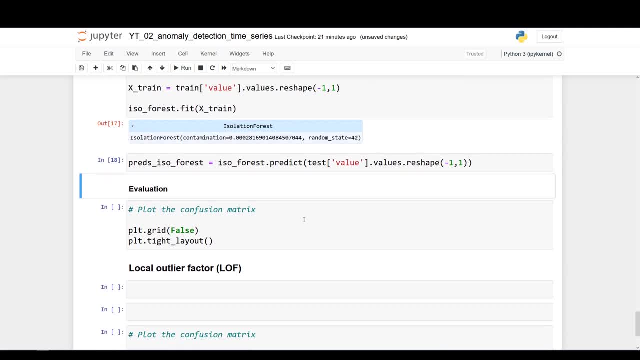 value dot, values dot reshape, And then here, minus one one, Perfect. So let's run this All right, And now it's just a matter of evaluating the model. Okay, So let's see if our model was able to identify this new anomaly, anomalous data point in the test set. 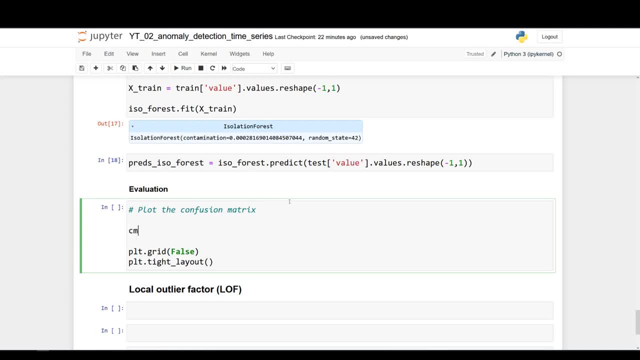 So confusion matrix, but only for the test set here. So just like before, cm is confusion matrix, Pass in your test is anomaly. and then your predictions: So Preds, isoforest, like so, And the labels again one and minus one, And then this cm is confusion matrix display. 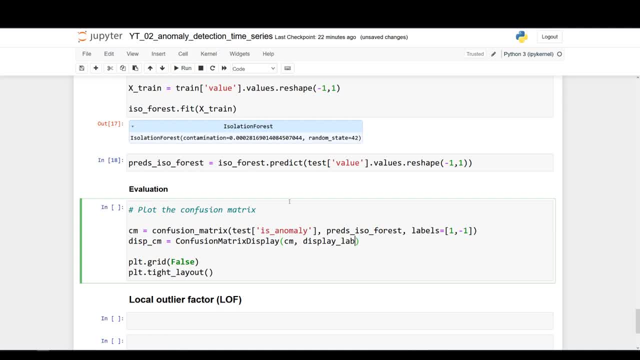 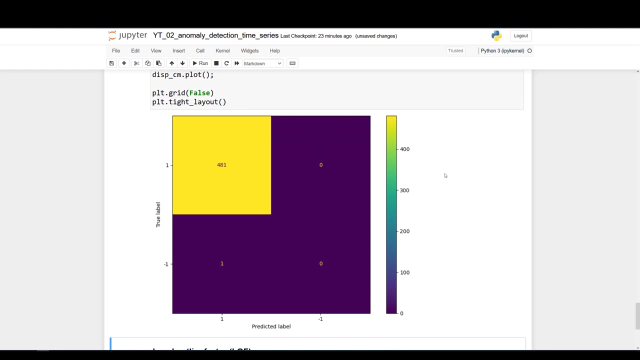 All right, cm display labels also one and minus one, All right. And then finally, we'll say that this cm outplot like so. So let's run this here, And I made a little mistake, I forgot my equal, Sorry about that- And you should get the following: So what do we see here? So, looking at, 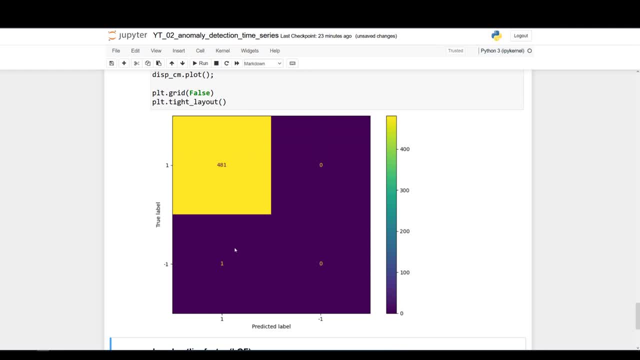 the confusion matrix, we can see that, in fact, it didn't manage to identify this new anomaly, right. So here we would expect to have a one at the bottom right, But it's not the case. In fact, the model only predicted that everything is an inlier, basically. So for the model, right. In the test set there are no anomalies when in fact there is only one. So that's why predicted label was one. So that's why predicted label is that default data goes to here instead of the stock. So the figure is still good. 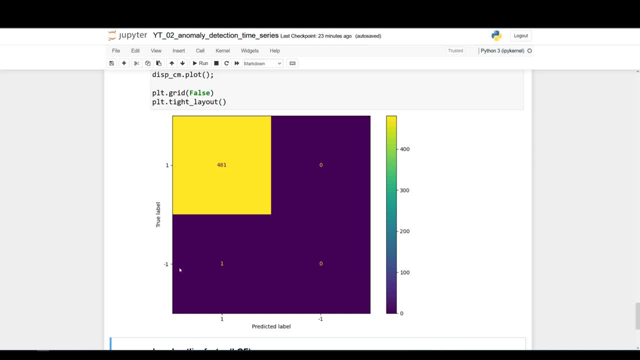 So that's why you know predicted label is one. In fact the model didn't storytelling yet, But it will. fundamentally. doctor dot Did the test set have one. so that's why you know predicted label was one, but the true label is minus one. so in this, 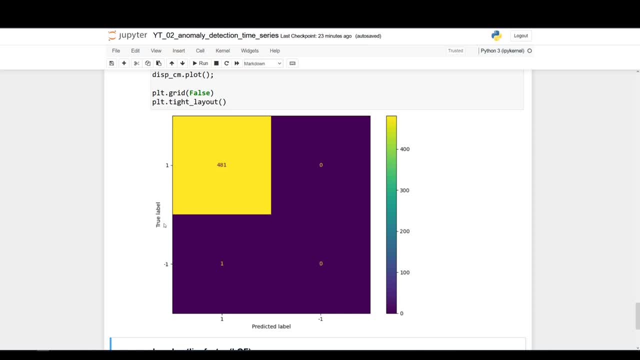 case, isolation forest did not manage to find this new outlier in the data, so that's it for this model here. let's go back into the slide, learn about the local outlier factor, and then we'll come back into the code so that we can implement it in python. all right, and now let's take a look. 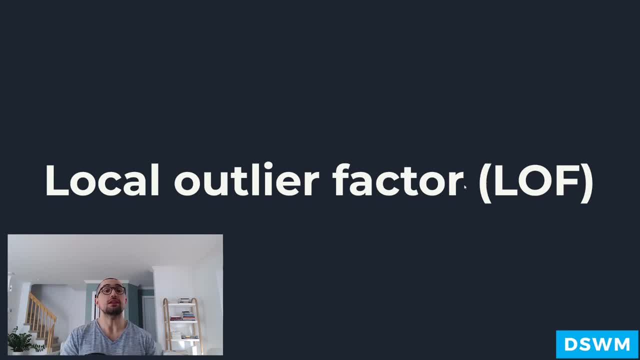 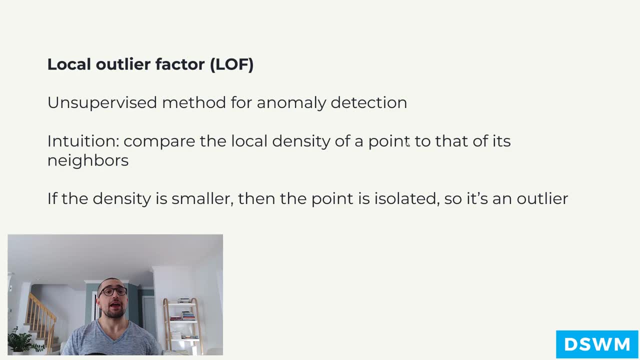 at the last method that we will explore today, which is the local outlier factor. so this is an unsupervised method for anomaly detection, and the intuition behind this method is that we will compare the local density of a point to the local densities of its neighbors, and so if the density is smaller for that point, then the point is likely to be isolated, and so 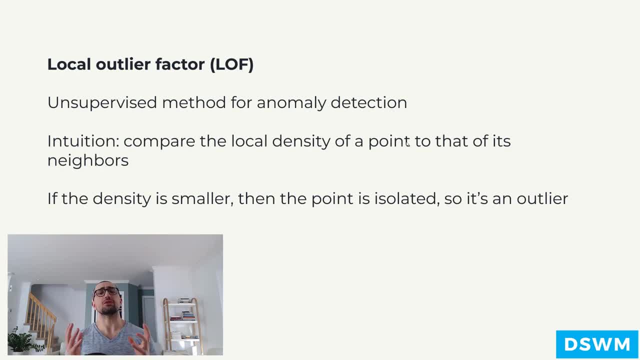 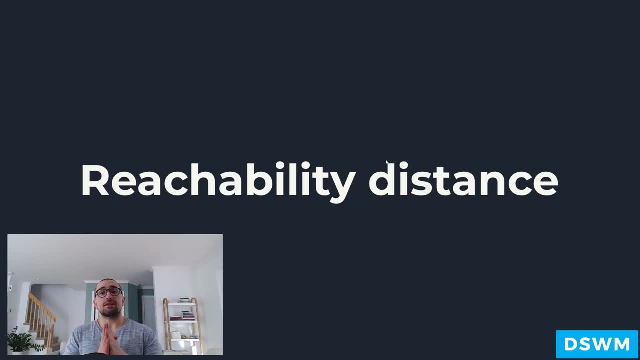 it must be an outlier. so that is really the general idea behind this algorithm. now, this is all based on a metric that is called the reachability distance, so let me do my best to explain to you what is the reachability distance. so let's take a look at. 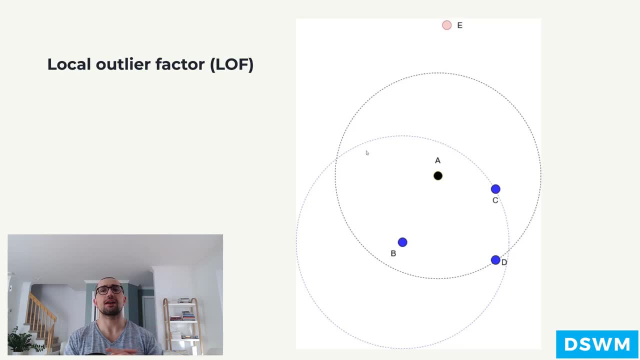 this picture here. okay, so here suppose that we are looking to compute the local outlier factor of point a and you set the number of neighbors to three. okay, so in this case b, c and d are the three closest numbers to the point a, and point e is too far away, so we're not going to. 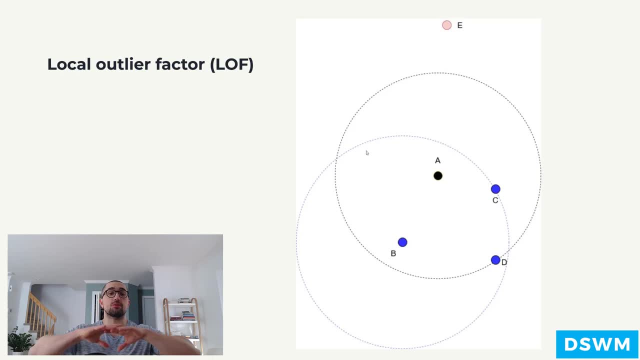 consider it okay. so what we'll do okay is that we draw a circle around point a. so point a is at the middle, is at the center of this circle, so we draw this black circle around, okay, um, and then the reachability distance is defined by this formula that you see here. okay, so it is the maximum. 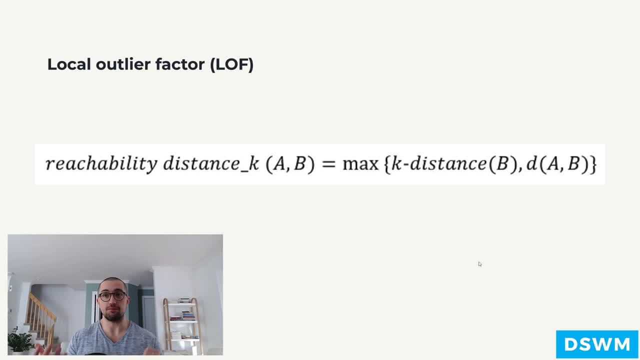 between either the key distance, uh, between the center of the circle and the center of the circle of b, so between a and b, or the distance between, or the actual distance, sorry, between a and b. now, the k distance of b, it is simply the distance from point b to its third nearest neighbor, and 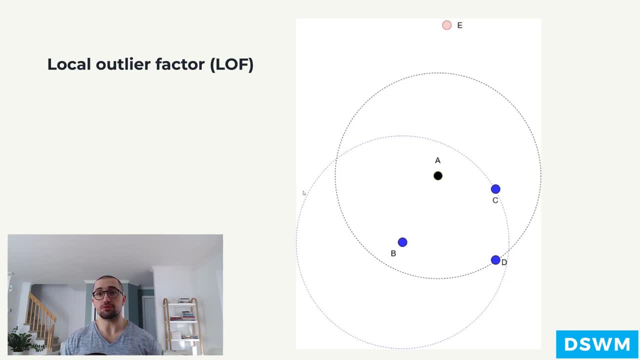 that's why in this figure right i have another blue circle here with the point b at its center to calculate that k distance of b. so what is the distance from b to its third nearest neighbor? so in this case it would be: c is the third nearest neighbor right. that's why c is on the edge of this. 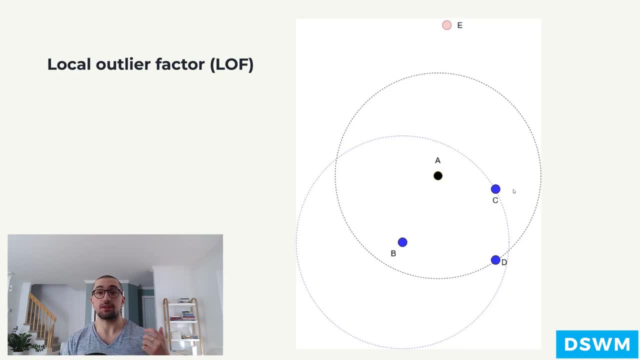 circle. so to calculate the reachability distance between a and b, you would take the maximum value, either between the distance from b to c or the distance from a to b. okay, and you take the maximum value of that and then, once you have that reachability distance calculated for all k nearest. 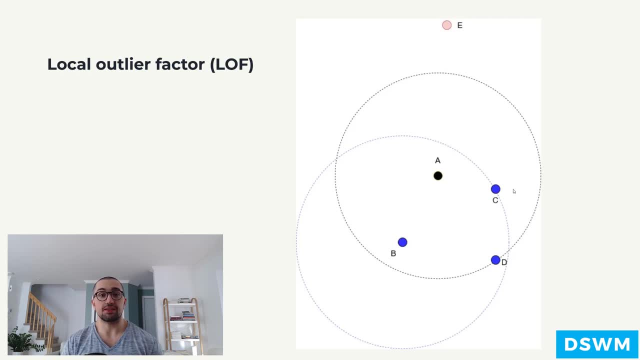 neighbors of a. you can calculate the reachability density, and that's simply the inverse of the average of all the reachability distances. okay, and so, intuitively, what the reachability density tells us is: how far do we have to travel to reach a neighboring point? right, and so if the density is large, then the points are closer. 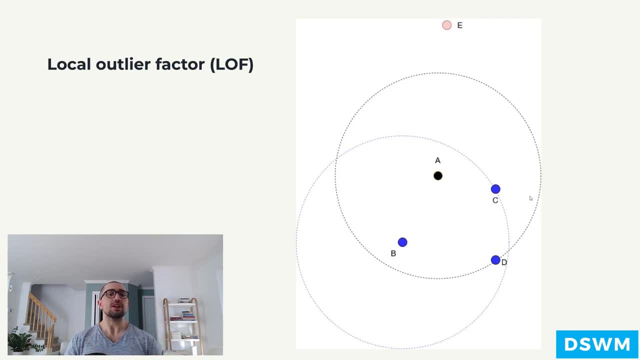 together and we don't have to travel for long, okay. and then the local outlier factor. it's simply a ratio of the local reachability densities, okay. so if we set k to 3, we will have three different ratios, right, and then we would average them and this allows us to compare the local density of 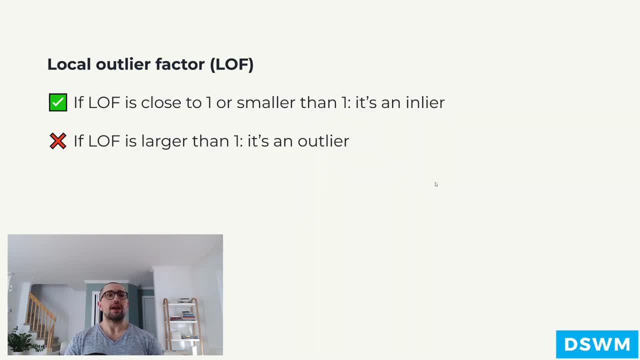 a point to its neighbors. and now, how do we identify, you know, if the lof is representative of an inlier and outlier. well, if it is close to one or smaller than one, then we conclude that it is an inlier. otherwise, if the lof is larger than one, then it is an outlier. 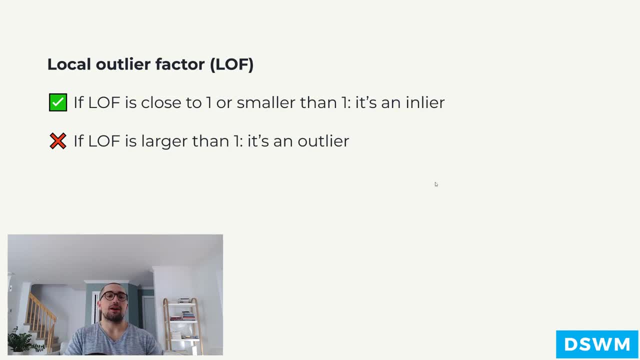 you, um, but this has some drawbacks right. uh, what does it mean? smaller, larger, right? uh, is an lof of 1.1. does that mean, uh, it is an inlier or is it an outlier, right, is it like larger enough than one or not really? so, uh, it has some drawbacks, right, and it really depends. 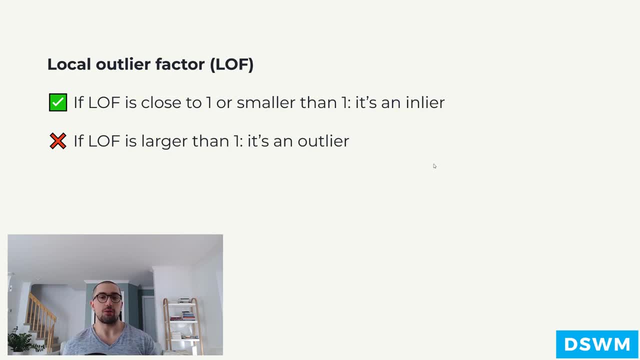 on the data set right. sometimes it's going to work very well. sometimes it's not going to work that well. it also depends you know how far away your outliers are from the normal data. so that's it for this method, and this is the last method. i will take a look at it today. 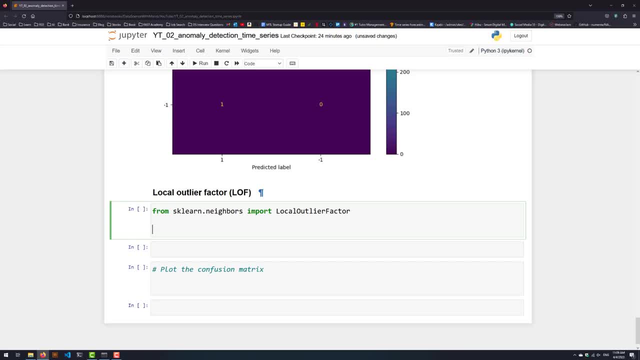 so let's go back into the code and actually implement it. okay, so last method that we are going to implement in this lesson is the local outlier factor. so again, a model that you can import from scikit-learn, so from sklearnneighbors. we'll import the local outlier factor and then 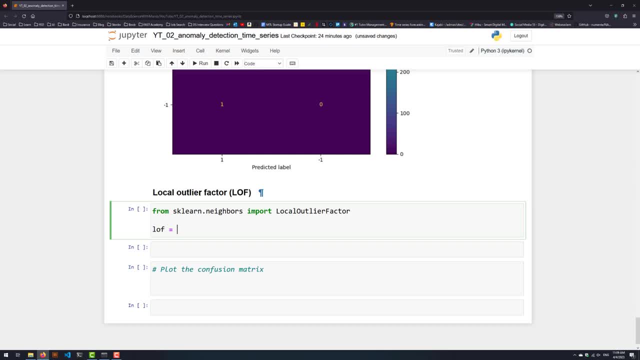 very simple, works pretty much the same way as the previous model. so lof is local outlier factor. also set the contamination level here. so contamination is contamination and here we need to set novelty. novelty equals to true, because in this case, uh, this is not necessarily anomaly detection. 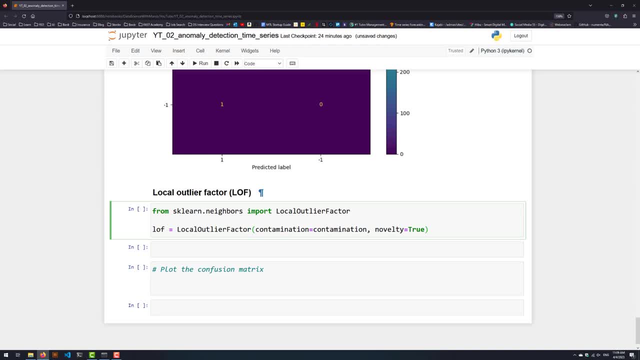 it is technically novelty detection right, because we are fitting on some data and then asking the model to predict on new data if we have anomalies or not. so anyway, uh, be careful with this right. if you want to use the predict method of local outlier factor, you need to set novelty equal to 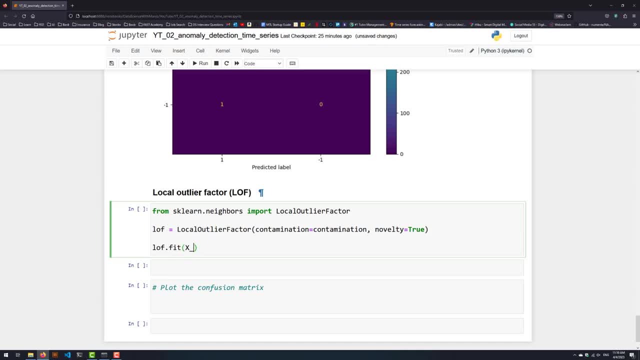 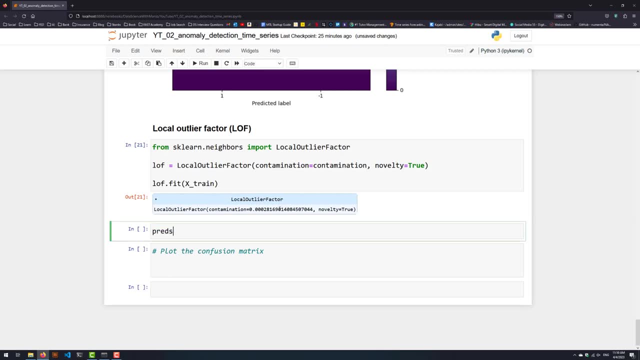 true. so, with that being said, now we can fit the model on our training data like so perfect, and then again just make your predictions so preds: lof is equal to lof, dot predict. and then you pass in your test value, dot values, sorry values. we shape minus one one, all right. and then, once you have your 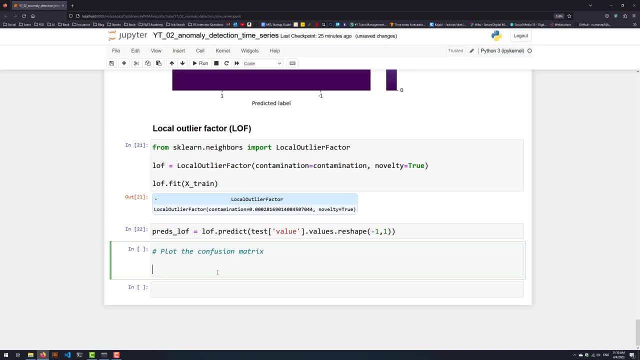 so if you have your predictions, uh, you are going to also want to put in the fact that you're going. and then, once you have your predictions, uh, you are going plot your confusion matrix. so cm is equal to confusion matrix, and then test is anomaly like so: 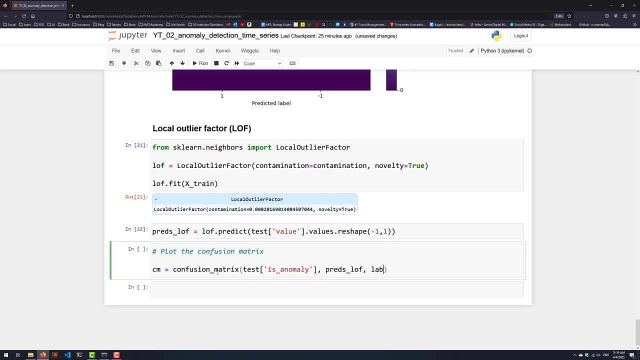 and then preds coming from the local outlier factor labels is again one and minus one, like so. and then this: oops, this cm is equal to the confusion matrix. display passing your confusion matrix and then display labels is also equal to one and minus one, and then it's just a matter of displaying it. so this cm dot plot like so, and you should get the following: 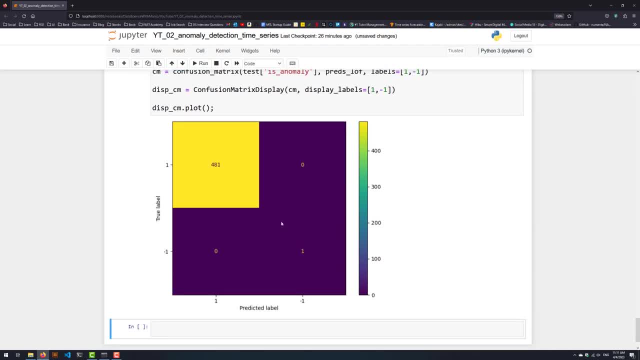 uh. so, as you can see now, very interesting, because local outlier factor was able to identify, uh, this, um, you know, incoming anomaly in the data set. so, as you can see, now we have a perfect confusion matrix, right, uh, everything. uh, so here's zero and zero at the top right and bottom left. so this is exactly what you want to see.